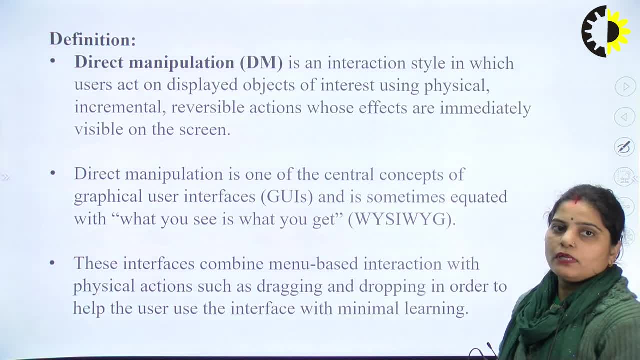 to discuss in front of you all. So, basically, first of all, I want to tell you about the basic definition that what is the direct manipulation? So? so, just like in a interface or when we are using interfaces, So direct manipulation is just like in technique, which is basically used to, which is basically: 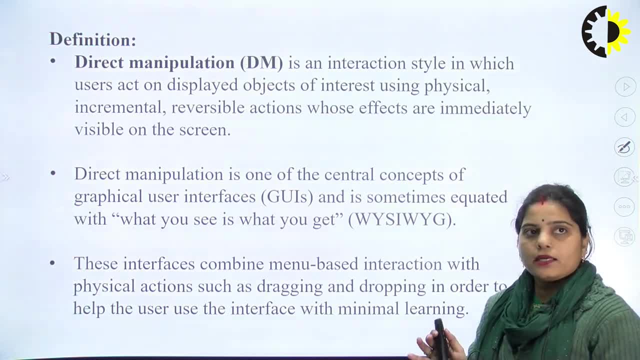 used as a interaction style in which user acts as an user, acts with their physical actions or it acts on the displayed objects of their interest using the physical, incremental or reversible actions whose effects you can see immediately over the screens. So basically, direct manipulation is a technique or it is an interaction style in which direct manipulation 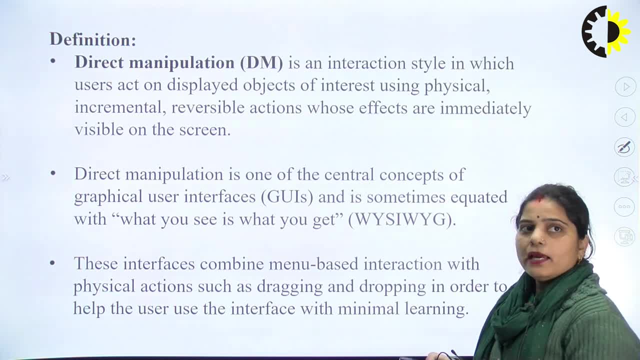 or any kind of users acts on the displayed objects which are displaying over the screen of their interest, with the use of their physical incremental, reversible actions and after performing the particular actions, that the effects of these actions can be seen immediately over the screen. So it is one of the central concepts of GUI's graphical user interfaces and also sometimes it is a similar or it is equivalent to the to the GUI's graphical user interfaces. So it is one of the central concepts of GUI's graphical user interfaces and also sometimes it is a similar or it is equivalent to the to the GUI's graphical user interfaces. So 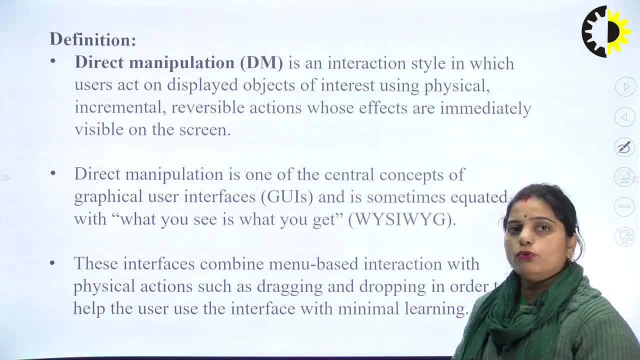 the word, just like here it is written at: what is what you see is what you get. So, similarly, just like in, what you see is what you get, direct manipulation is also a technique in which you applied or you with the use of the physical actions or with the use of the. 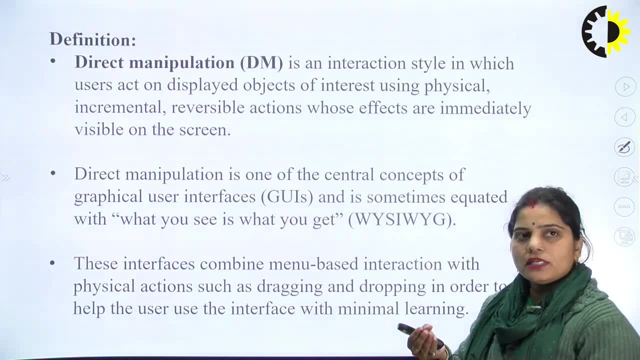 reversible or incremental actions. you can. you can manipulate the things directly which you are seeing over the screen and the effects can be immediately seen or observed over the screen. only The interfaces, which these interfaces when combined with the menu based GUI's graphical organisation and the interface which these interfaces when combined with the menu based. 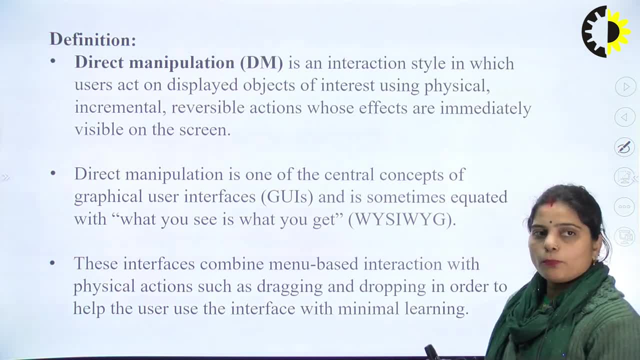 interaction with these physical actions, just like dragging and dropping in order to help the user's in performing the interfaces. that kind of learning involves the. that kind of of that kind of learning involves the. that kind of technical involves the minimum learning, here the user. that kind of technique involves the minimum learning, here the user does not. 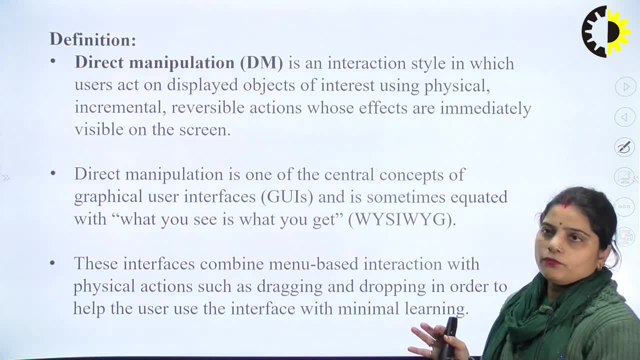 need to learn more the things, only what. what he or he or she has to do. he has to, he or she has to depend over only on the physical action. So Convincing Guest Toentist floss has to stand alone in that context of in engagement with body. this one, sort of an example to know how to stay away form one Claraی another. so the direct Нов Longanimость apps, and this is similar to you while looking for direction of only, and that's why that, as shown, may be going for direction, all this via the sabemais. 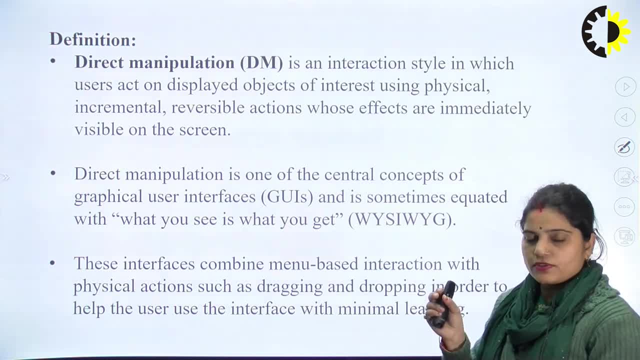 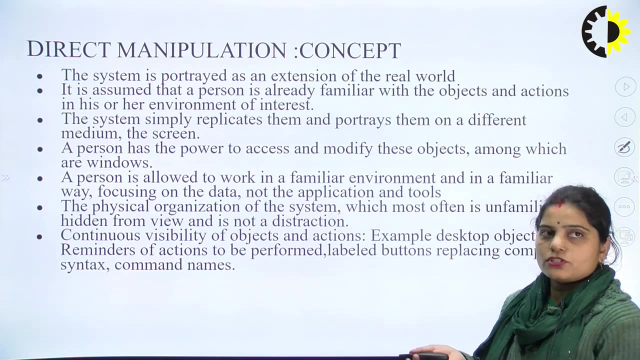 another, So directly with the use of, with the use of these physical actions, they can manipulate the things over the screens which are properly or which are easily visible over the screens. Now the concept behind the direct manipulation is: it is just like in the system which is: 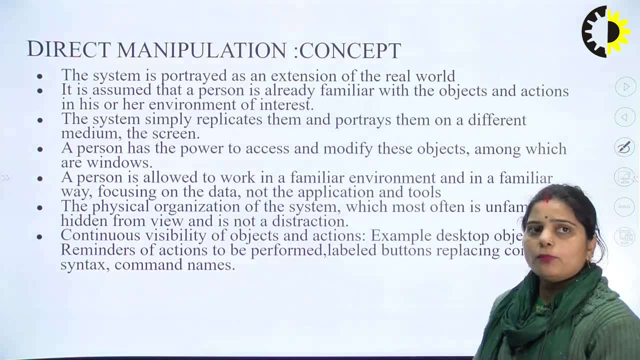 portrayed just like the extension of the real words. So in direct manipulation, it is assumed that the person is already a familiar with these objects or with these actions. whatever the actions or whatever the things are are running over the environment, his or her environment of interest. 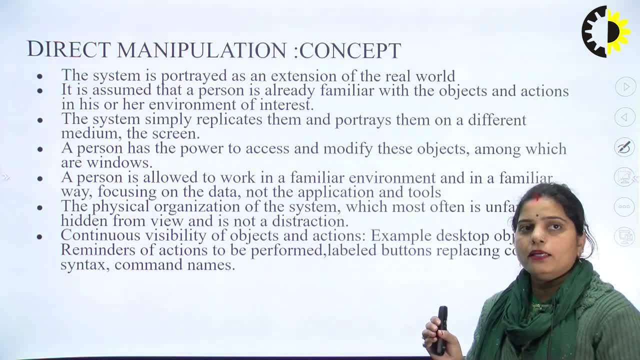 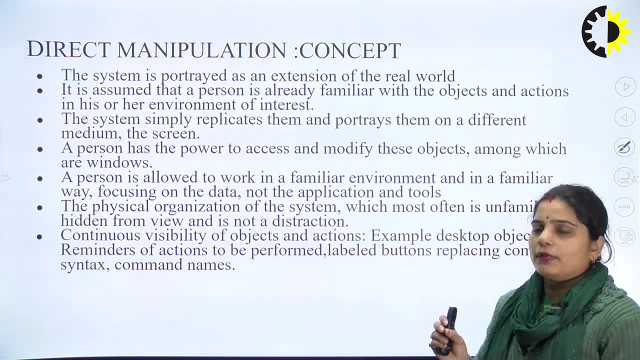 So these things or these environments are already known to that person. So the direct manipulation concept is basically that that the system simply replicates them and portrays them on a different medium, which is the screen here. only So if a person has the power to access or modifies these objects, among which objects 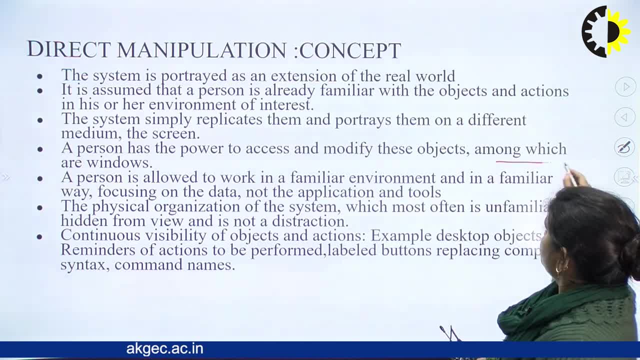 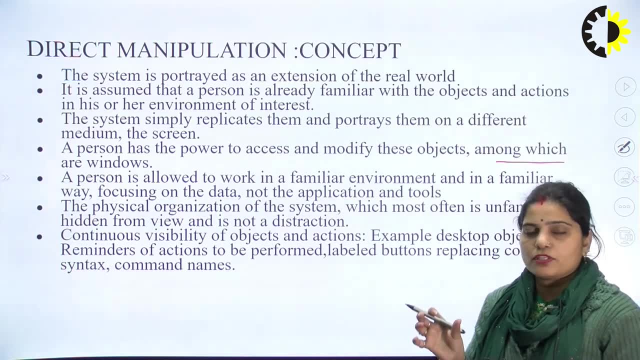 among which are the windows only. these are the windows over which the user can access or modify these objects which are visible over the screens or which visible over the windows. So here the person is allowed to work in this familiar environment and in a very much. 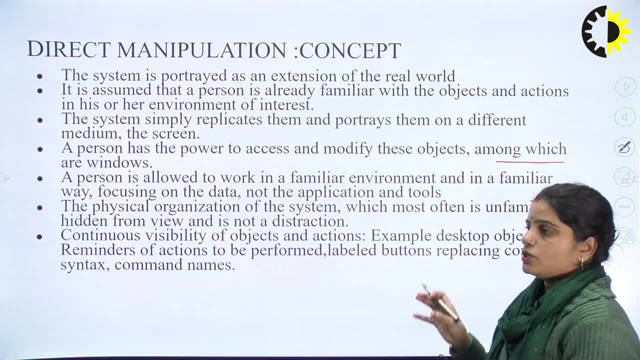 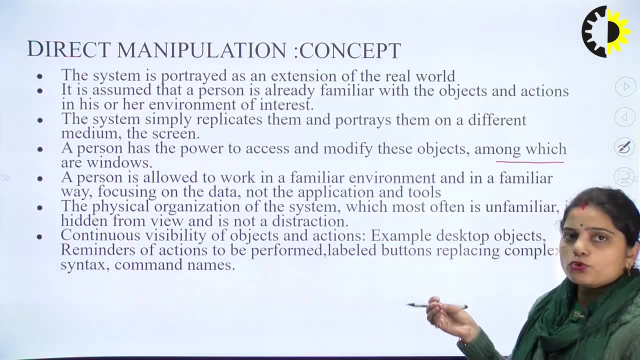 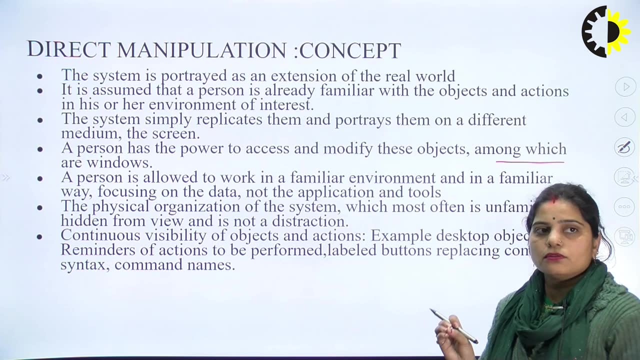 familiar way, focusing only on the data, not on the applications or the tool palettes here only. So the basically, what is the physical organization of the system, which is most often is unfamiliar? generally, what happens? Say that the physical organization of the system is not known to the users, or it is. 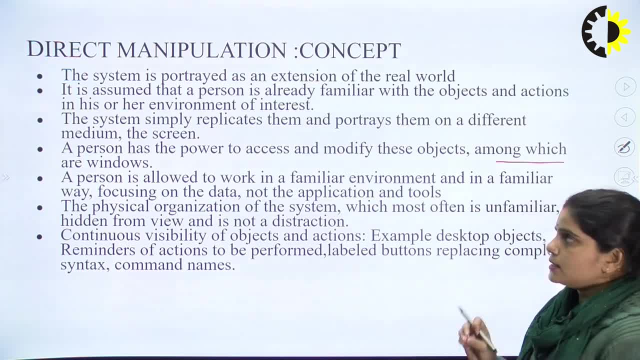 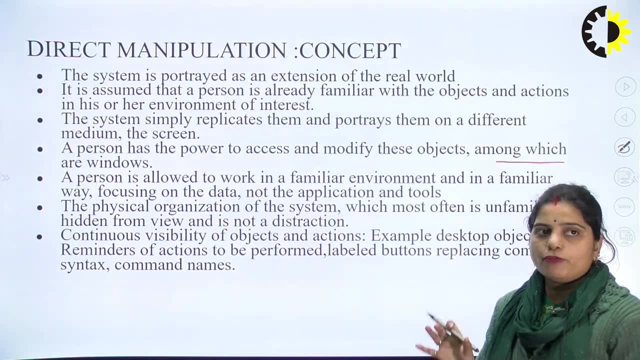 in the hidden form. So, basically, this concept is helpful in those concepts only where the physical organization of the system is unfamiliar or hidden from the view. So with the use of these, with the use of this technique, one can easily perform the physical actions and can view the objects and can manipulate it as per his or her requirement. 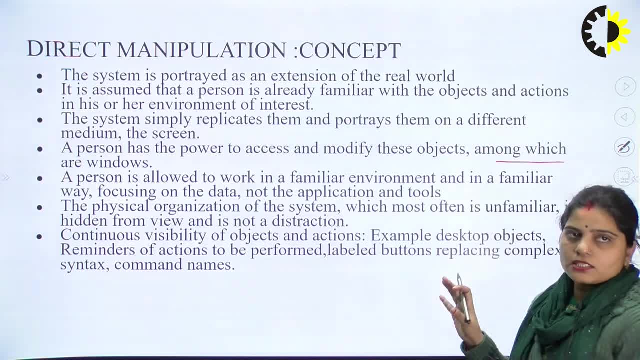 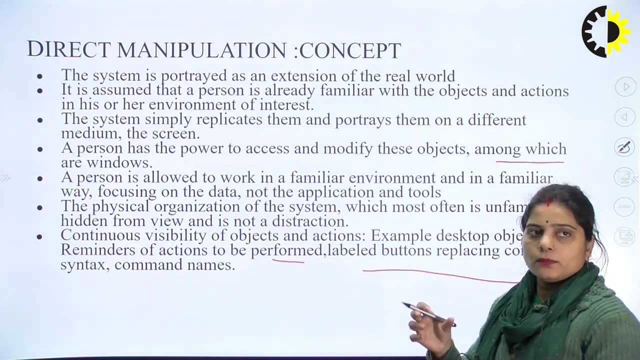 only Consider things easily. Consider tools also, or actions. here we can see, just like desktop objects, reminders of actions to be performed, label buttons replacing the complexity or replacing the complex syntax or commands name. so these, these are the basic concept behind the direct manipulation techniques, just just like 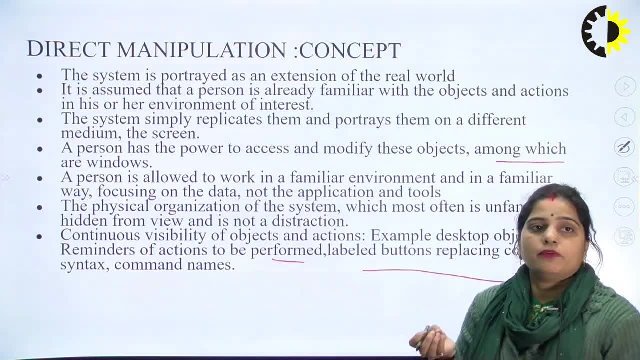 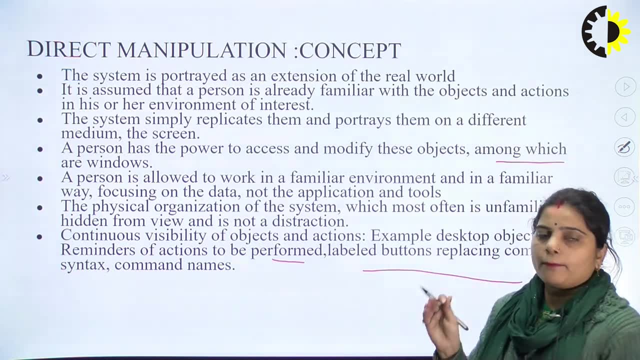 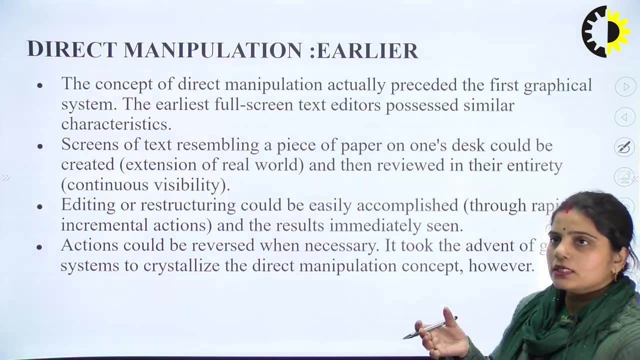 when it, when it is useful, or when the continuous visibility of the objects or actions can be seen here. okay, so these are the some examples where we can apply the direct manipulation techniques. now this, what? what is the earlier concept behind the direct manipulation was, earlierly it was for forwarded behind the concept of graphical systems. so the director, the concept. 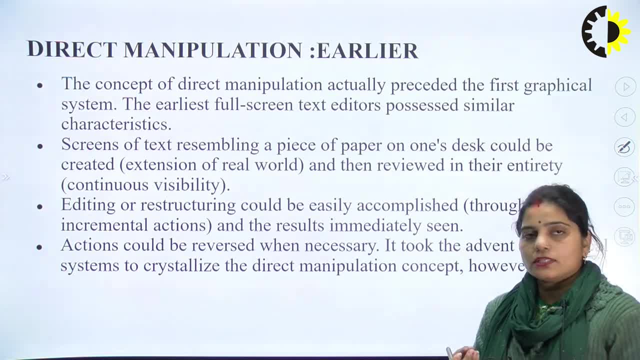 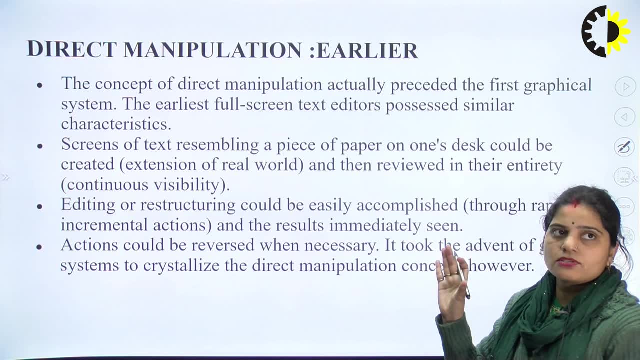 of direct manipulation is actually preceded the first graphical system. okay, so what? we have observed that the earliest full screen text editors possess the similar characteristics, just like the direct manipulations. what, uh? what was the concept in earlier? was that the screens of text resembling the piece of work, suppose piece of paper on one desk, and it should. 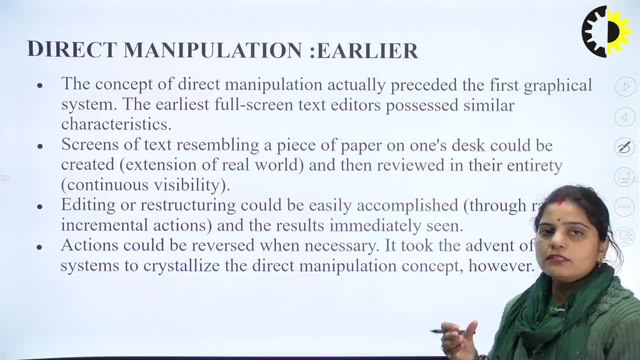 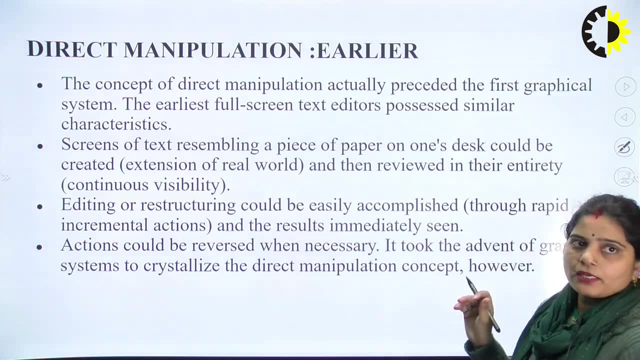 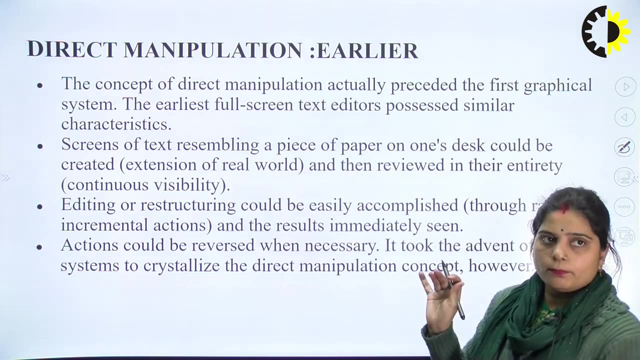 be created and then reviewed in their entirely continuous visibility. only now what happens? that editing or restructuring could be easily accomplished through the rapid incremental actions and the results will immediately be seen over the screens. only now actions also can be reversed when necessary, whenever there is a data retention function, so alive the search will not be. 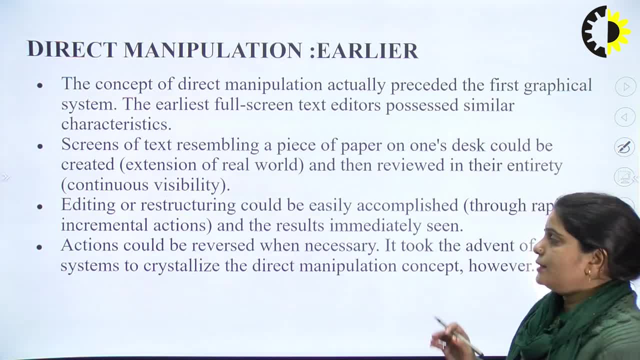 completely tenants, and whenever there was a requirement, then these actions could also be reversed, just like. suppose I did something wrong over the screen, So what alternative to that was that? that the option undo was also given here, So that actions can also be reversed whenever there is a requirement or whenever there is? 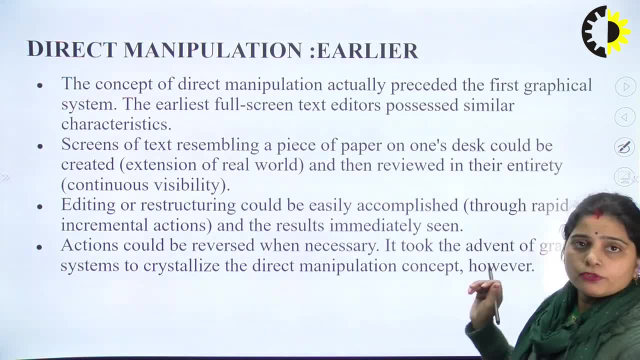 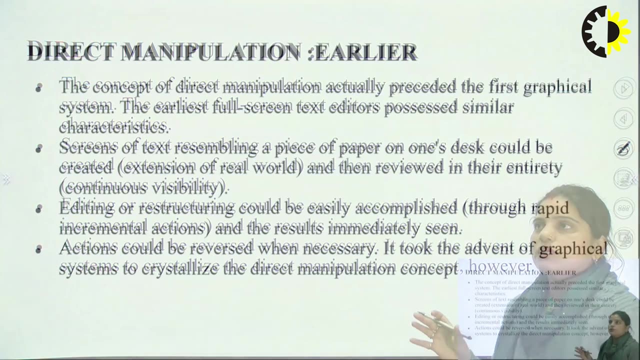 a necessity of that, things only. So it took the advent of graphical systems to crystallize the direct manipulation concept. however, basically the direct manipulation concept is used to crystallize these things, the advance of these graphical systems here. So that is why the direct manipulation concept or the direct manipulation technique is totally 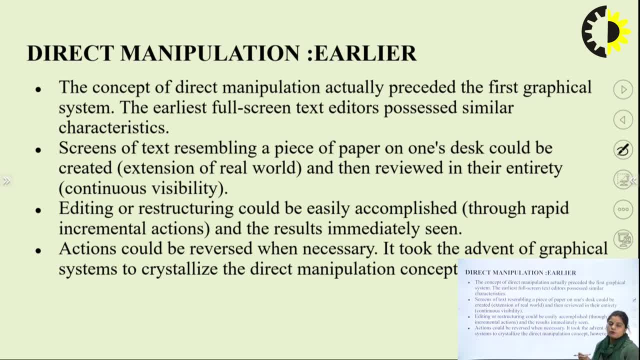 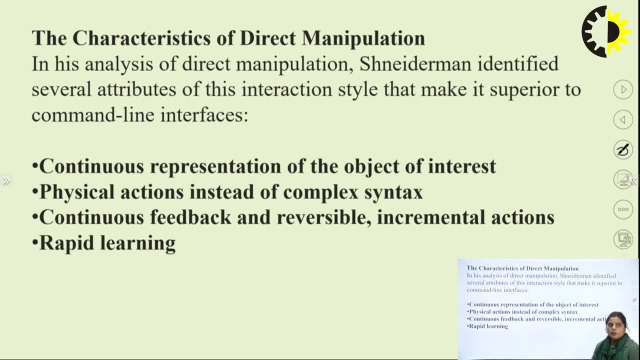 based on the physical actions or reversible or incremental actions of the user only. Now, what are the basic characteristics of the direct manipulation- The direct in this analysis of the direct manipulation. in his analysis he points out the basic characteristics of direct manipulations. 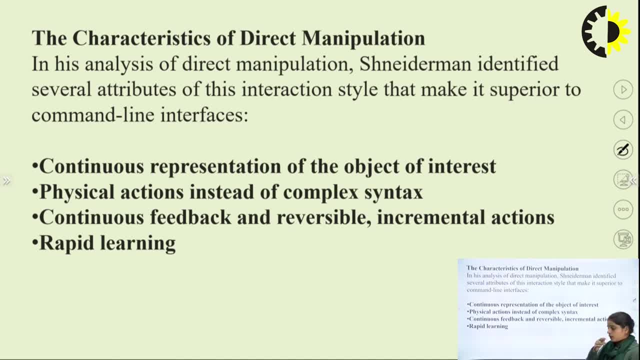 The senderman had already known about the senderman principles in human-computer interface. So one of the person, sender man has identified, just like the several attributes of this kind of interaction style which make it superior in comparison to the command line interfaces. So what these characteristics are, which sender man has identified it and which makes it different. 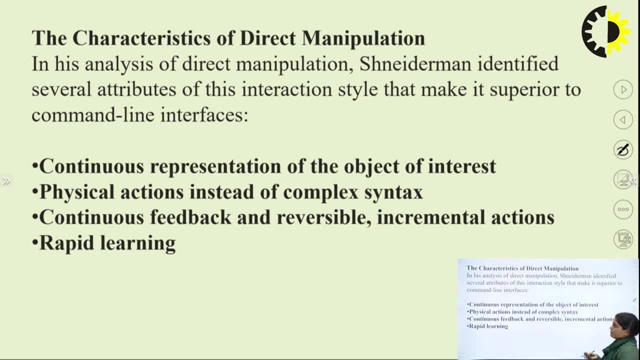 makes it superior in comparative to command line interfaces are: first is continuous representations of the objects of interest. whatever the objects of interest are they, they are continuously represented over the screen. second one is, instead of writing the complex syntax, or instead of remind, reminding the complex systems, here only what is required, here only the requirement. 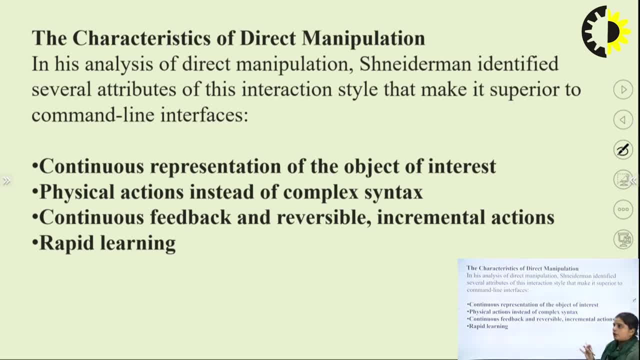 of physical actions is required here only. instead of that, complex syntaxes or instead of that, instead of reminding these kinds of complex syntax in your memories. next one is continuous feedback and reversible incremental actions are required here. and the last one is rapid learning. here is here nothing more than no complexes syntax has to be required. 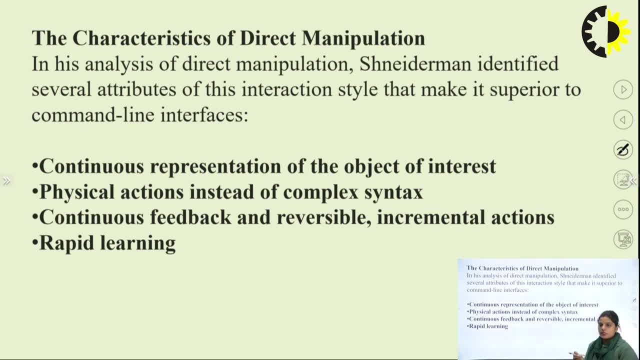 to learn here. whatever you are doing, if you are doing it first time, then you can learn again and again, and you can rapidly learn the things here only because there is no syntax required in any context, of context so denoting this. so that is what you have to learn now. so if you are done, you are done, then you have to do the next step. so here we do see that what we have- login screen here and at the end of the last table and the last example required. there is no complex syntax is required to learn. 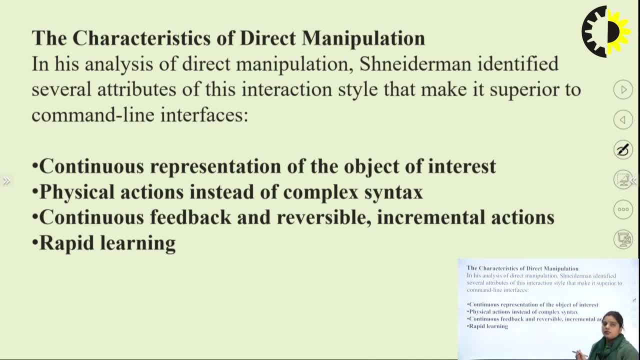 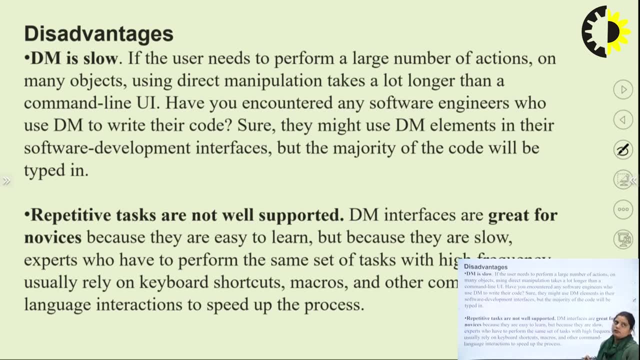 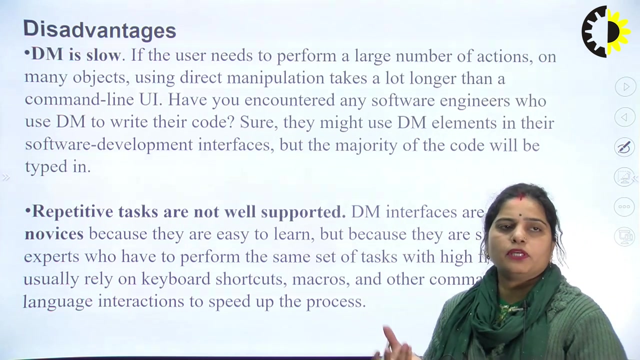 So the learning here, with the use of direct manipulation, the learning is rapid. only Now, here, apart from these characteristics, or apart from these advantages, here some disadvantages of direct manipulation is also discussed. First disadvantage is: direct manipulation is slow. Now how the direct manipulation technology is slow, the if suppose in some cases, or if 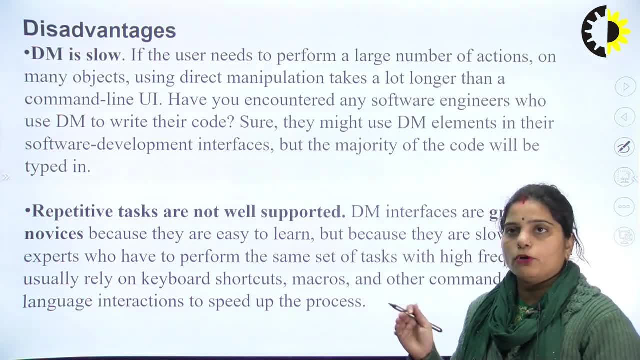 the user wants to perform a large number of actions on many objects. Suppose there are too many objects over the screen and if the user wants to perform the large number of actions on these objects with the use of direct manipulation techniques, So when? if the user is using the direct manipulation techniques to perform the large number of 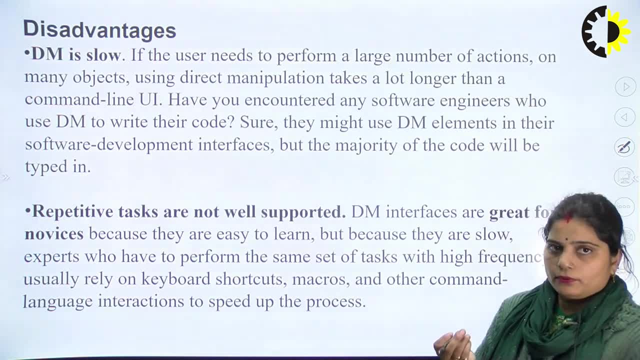 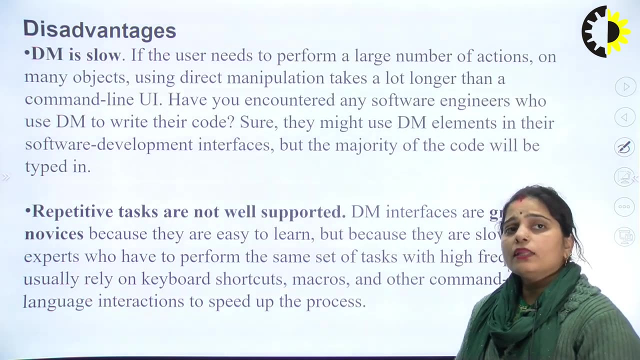 actions over the many objects, then the time taking process is too much long in comparison to the command line interfaces. So with the use of direct manipulation, With the use of direct manipulation techniques, it takes a lot longer time than a command line techniques. If you have just- like here it is written that- have you encountered any software engineers? 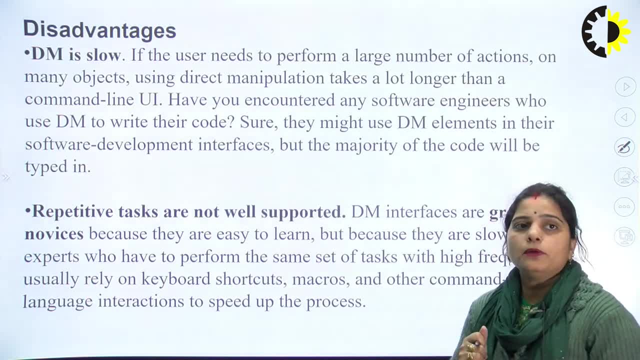 who used direct manipulation to write their code. Sure, they might use, they use the direct manipulation elements in their software development interfaces, but the majority of the code will be typed in ok. So what is observed here? that whenever there is a requirement, or whenever there is a requirement, 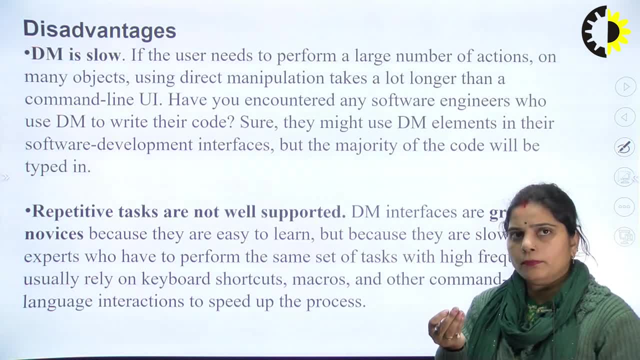 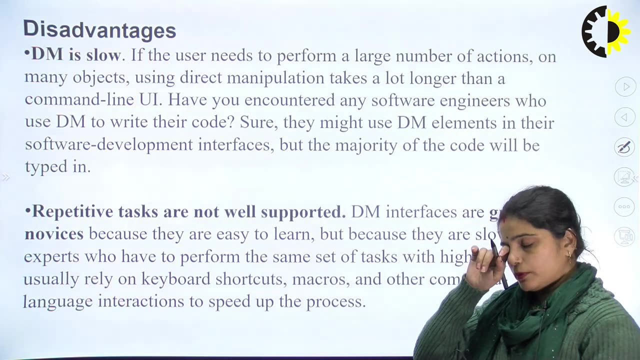 there is a requirement. Whenever there is a requirement of some actions to be performed over the object, then we can use the direct manipulation. But when there is a requirement of large number of actions, when there is a encounterment of large number of codes, then majority of the codes will be typed in. then we recommend: 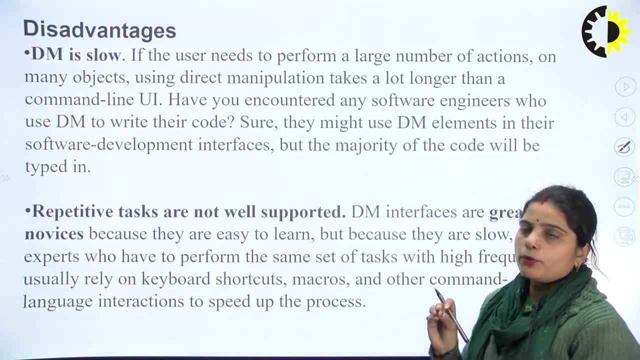 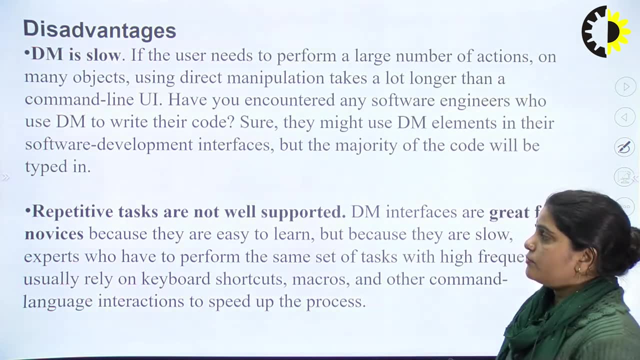 not to use the direct manipulation technique because the time process or the time taking or the time slot for the direct manipulation for the large number of actions will be too much. Next one is repetitive tasks are not well supported with the use of direct manipulation interfaces. these are great for novices because they are easy to learn. 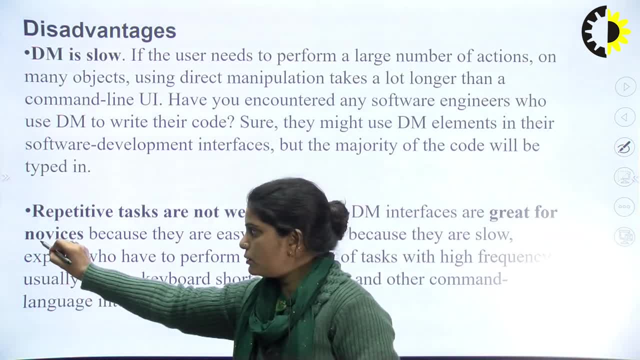 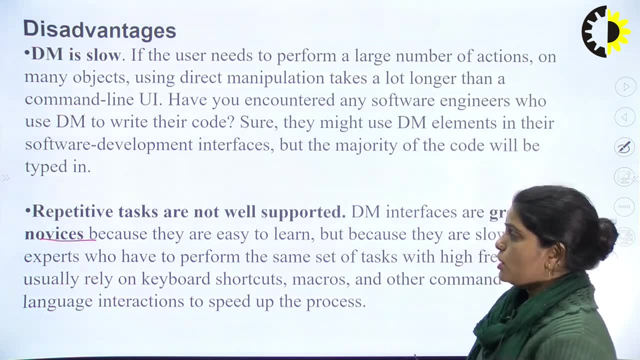 There are basically the word here is used- novice. so there are three kinds of users: first one is novice, then intermittent and the third one is expert user. So the novice users are the new users. or they are not well familiar with the systems, or they are not too much experienced. 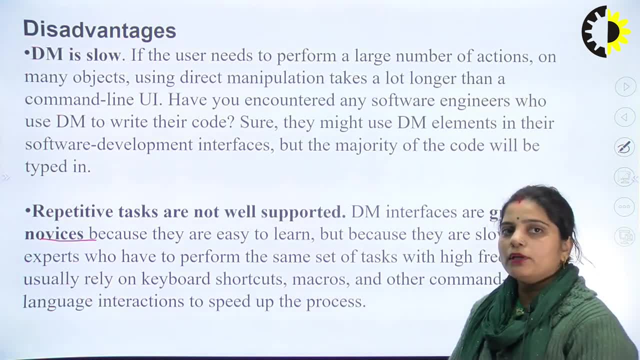 So let us see. So direct manipulation techniques or direct manipulation interfaces are great for that kind of users, for the new kind of users who are not very much experienced or who are not very much familiar with these things. So this technique is: this technique is great for supporting these kind of users, because 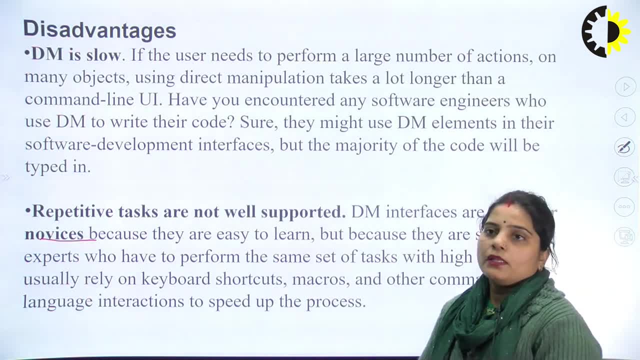 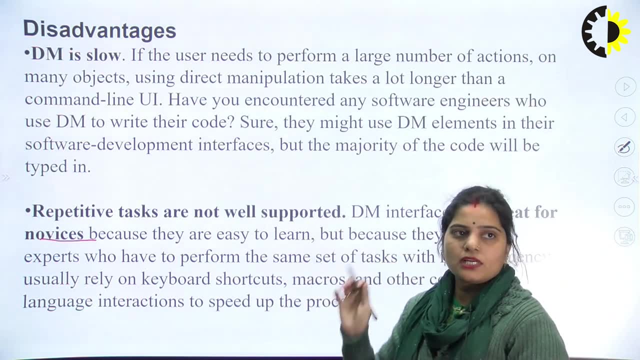 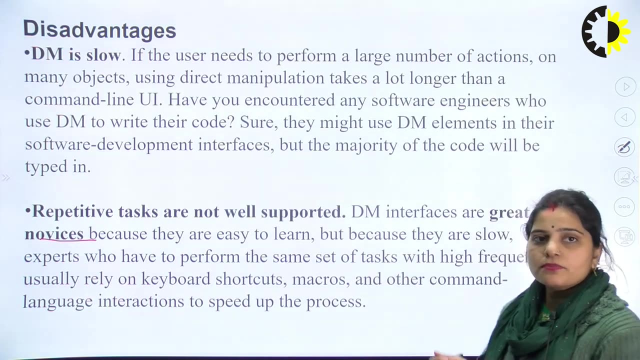 in this technique. there is no complex syntax to learn. there are no. there are not too much syntax to be remind in your mind. So this technique is easy to learn. So that is why it is great for novice users. But because they are slow, so for experts who have to perform the same set of task with 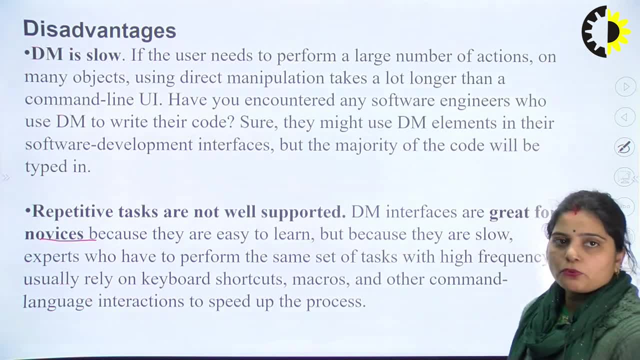 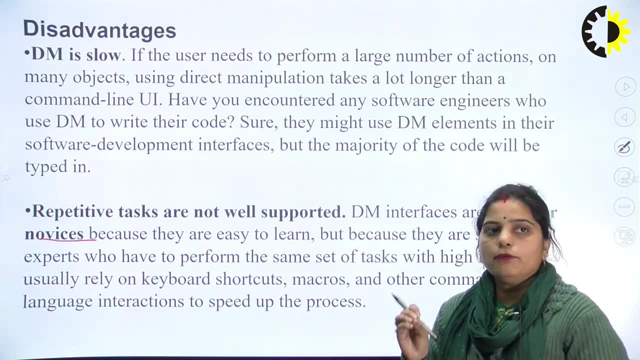 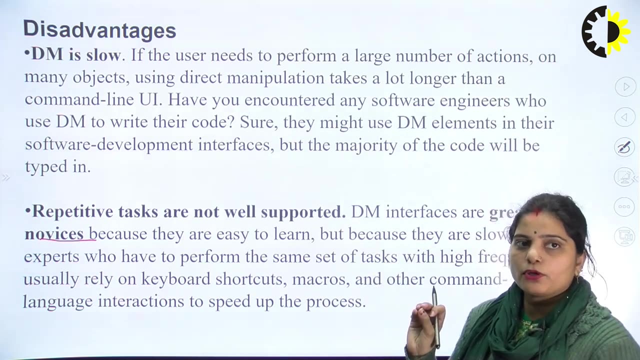 the high frequency, usually rely on the keyboard shortcuts, macros and other command language interactions to speed up the process. So for novice user this is good. but if there is a requirement or if this technique is used by expert, then they recommend for they recommend less for this technique because they have 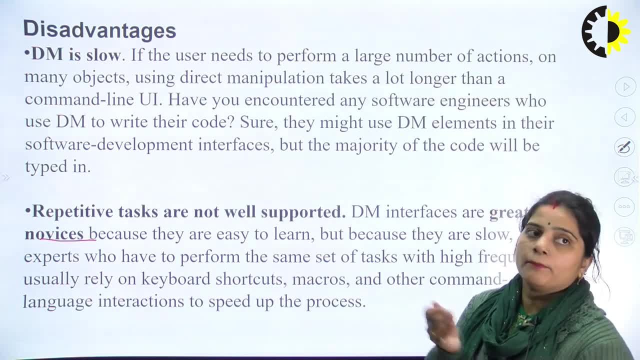 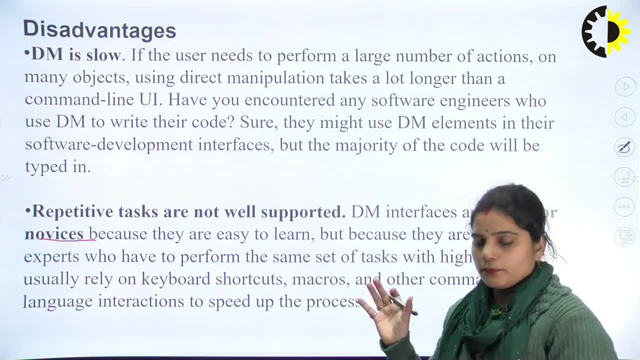 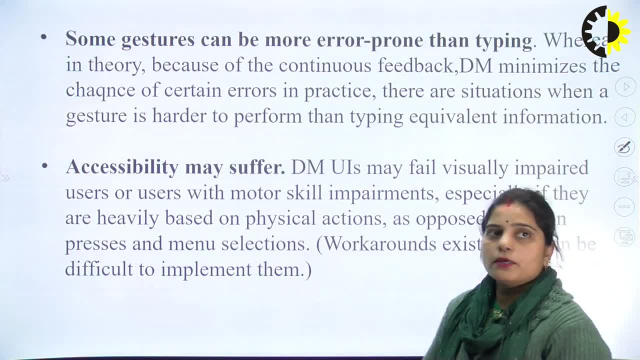 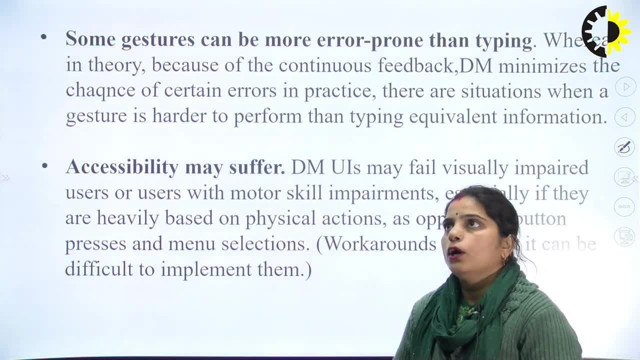 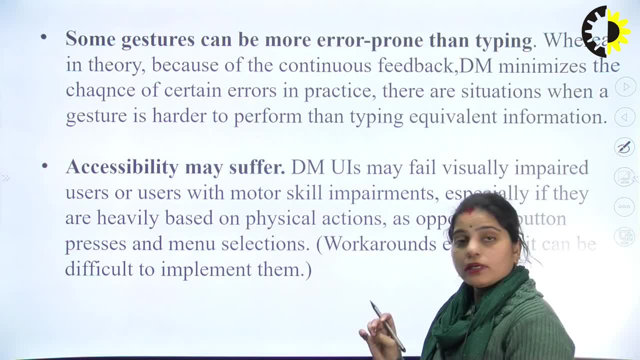 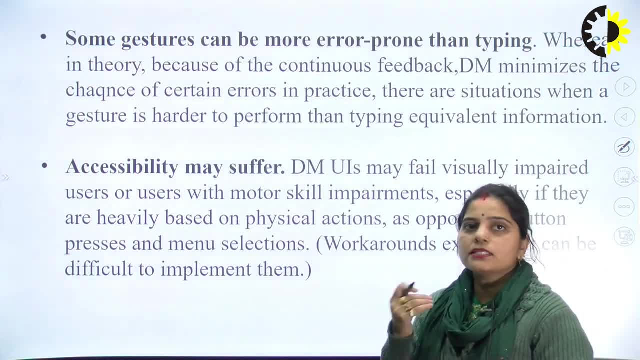 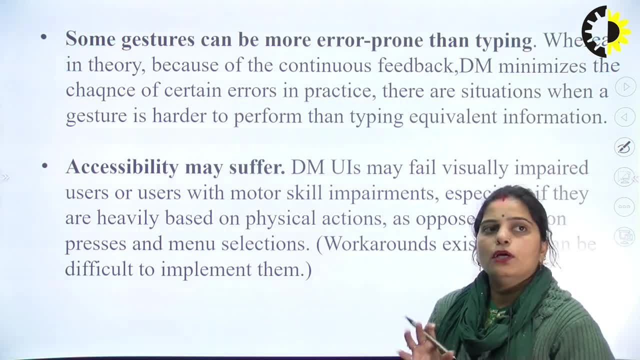 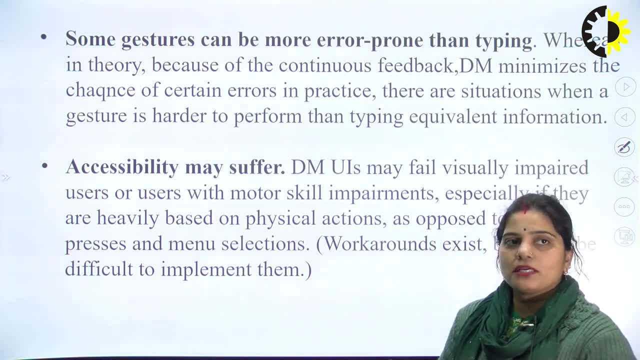 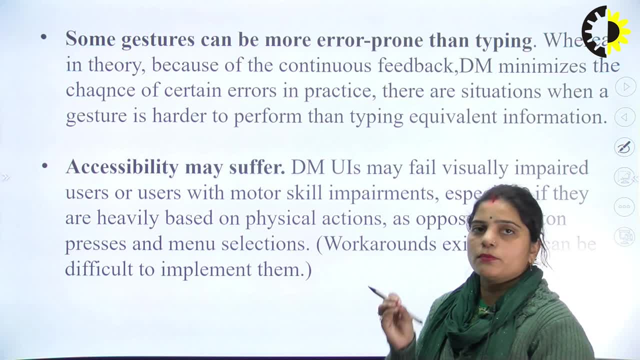 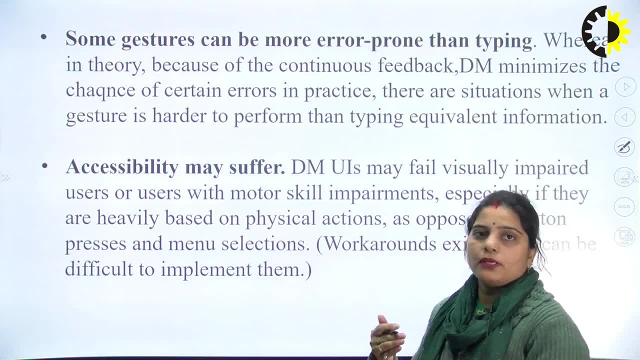 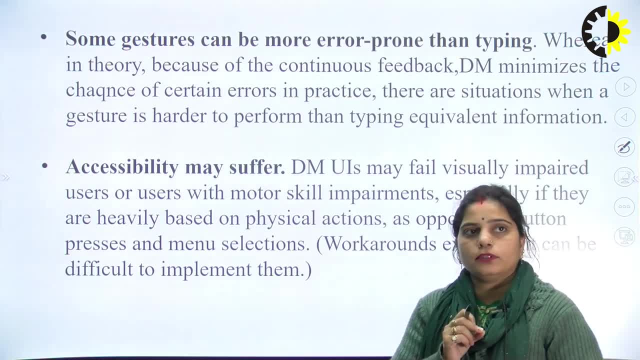 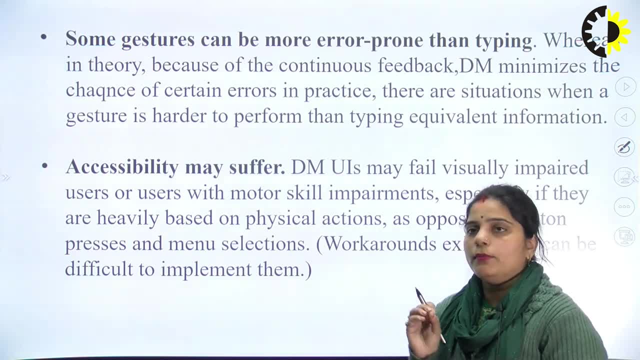 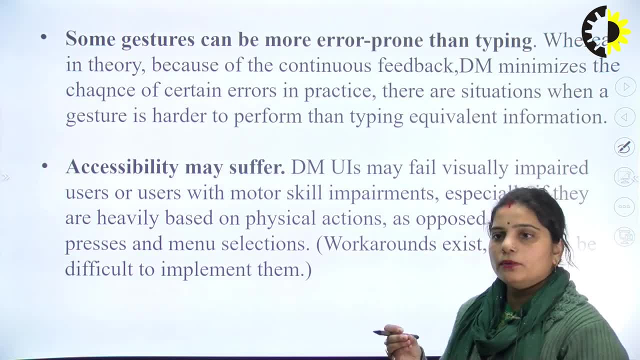 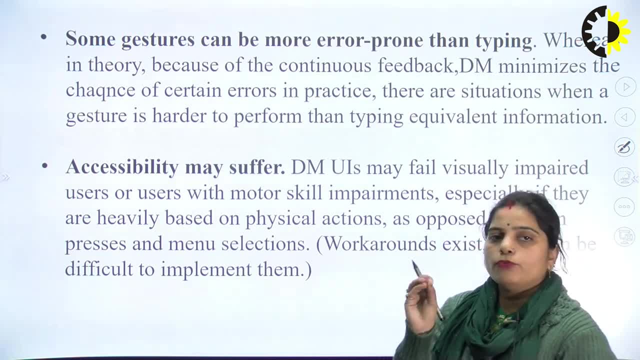 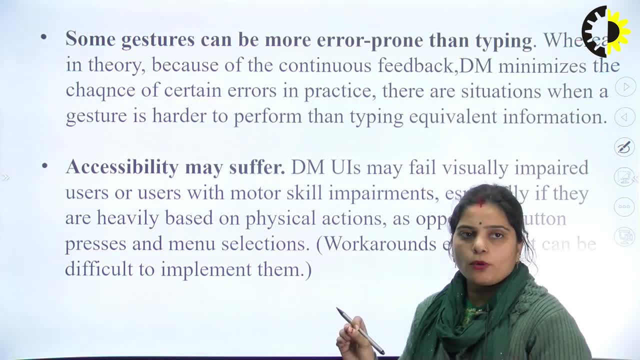 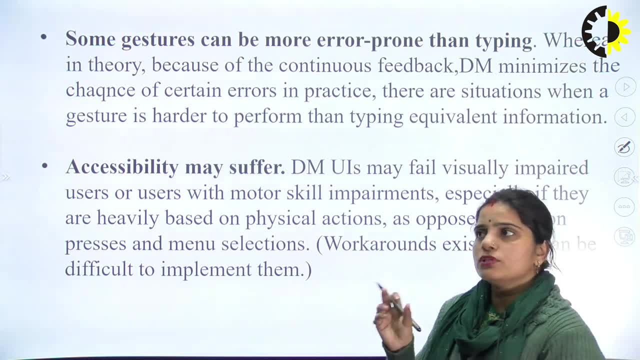 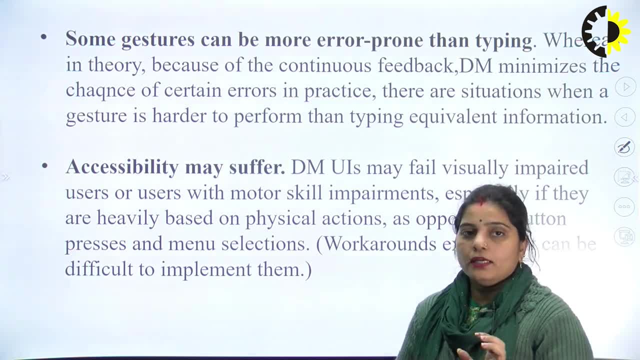 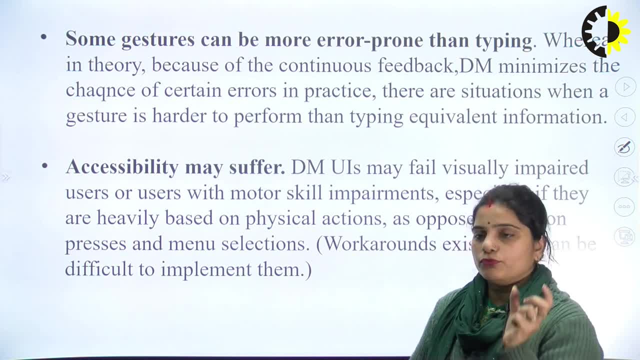 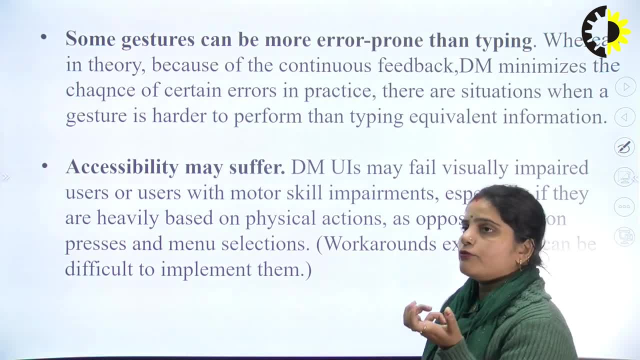 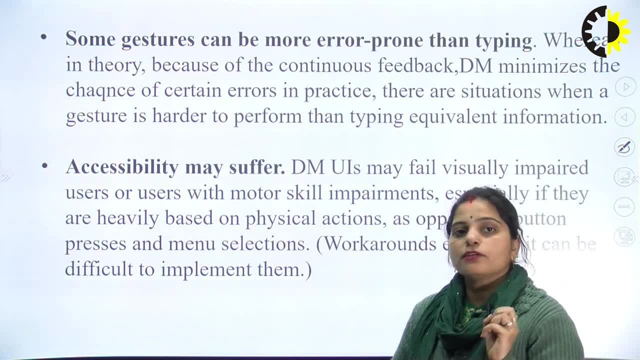 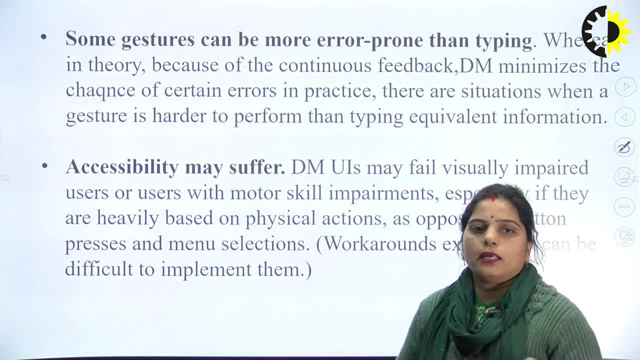 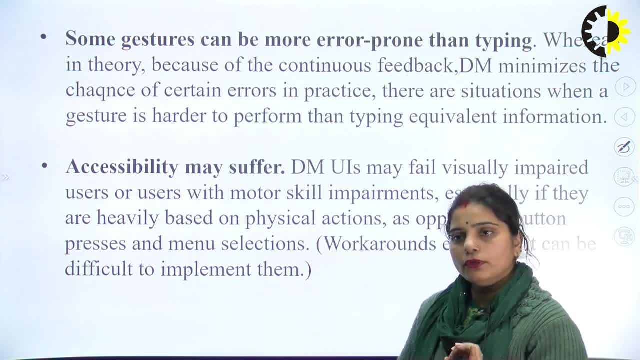 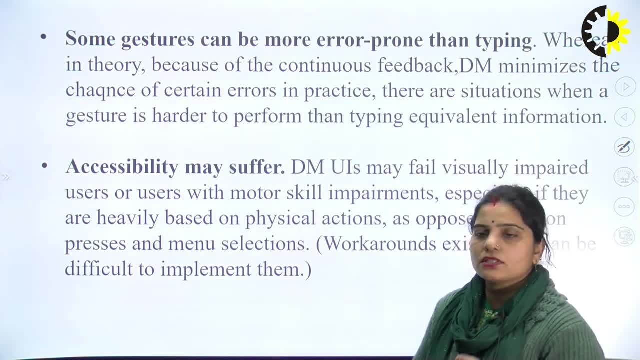 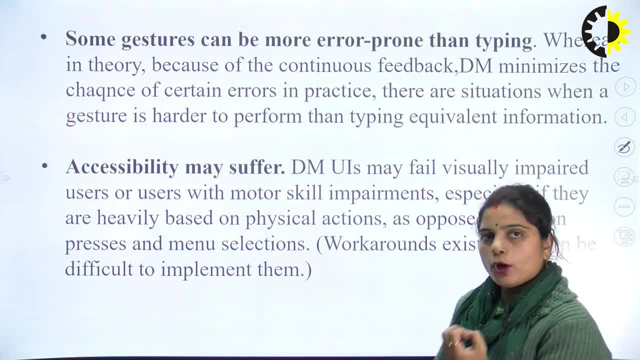 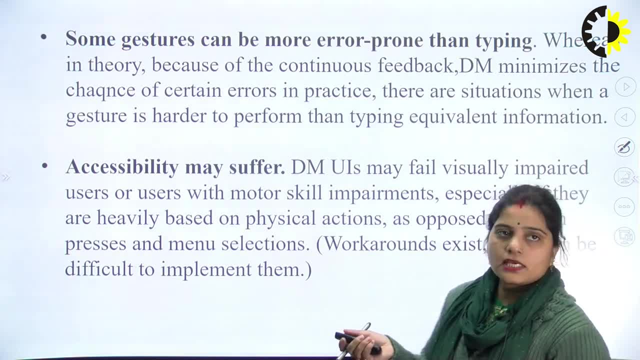 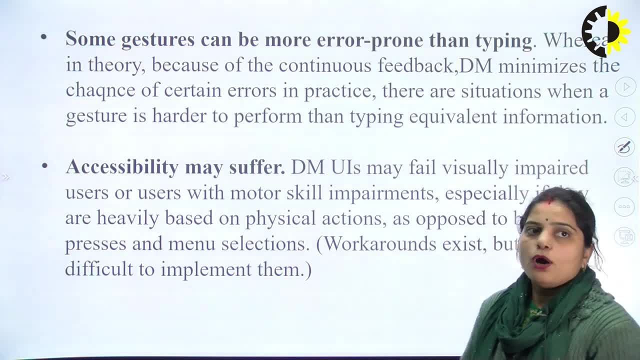 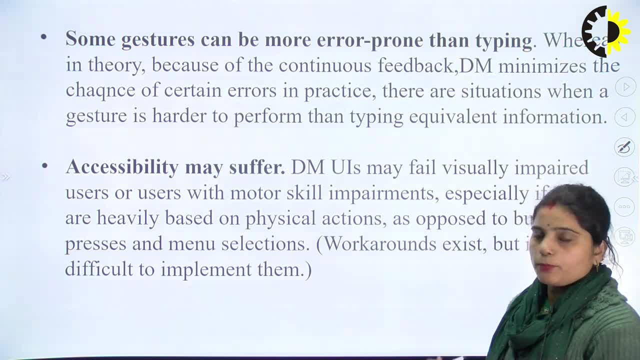 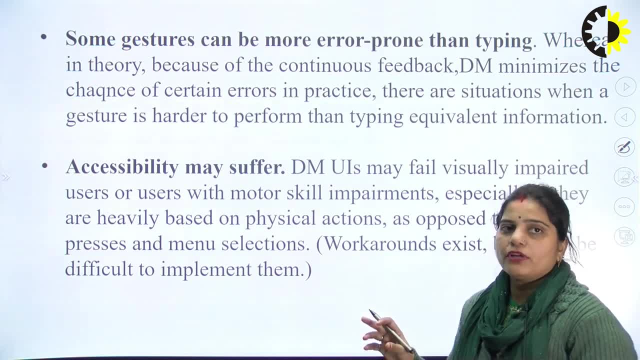 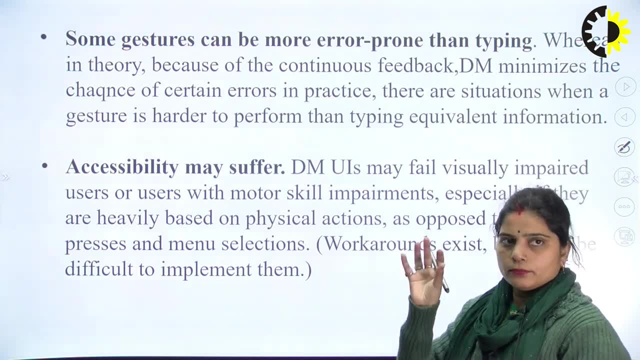 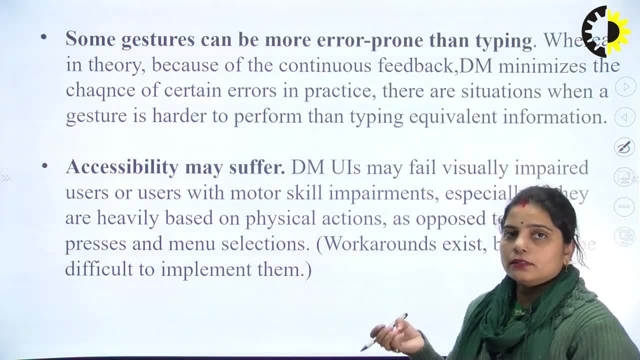 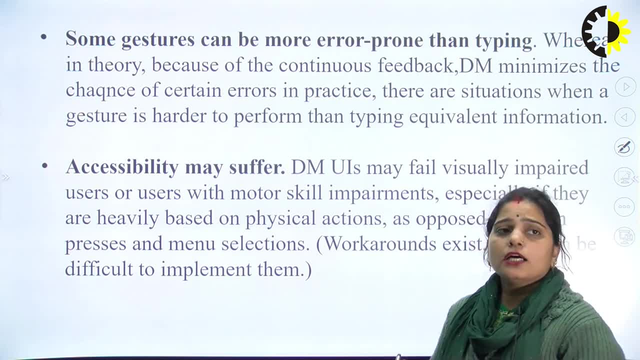 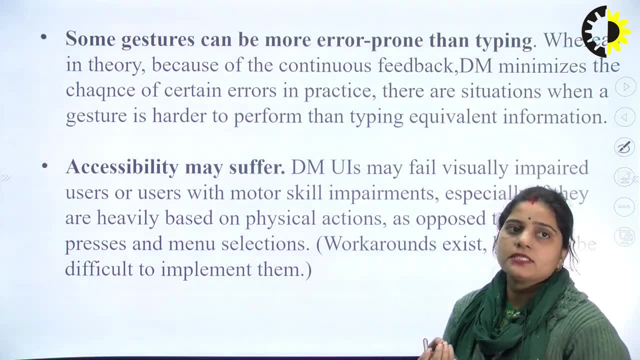 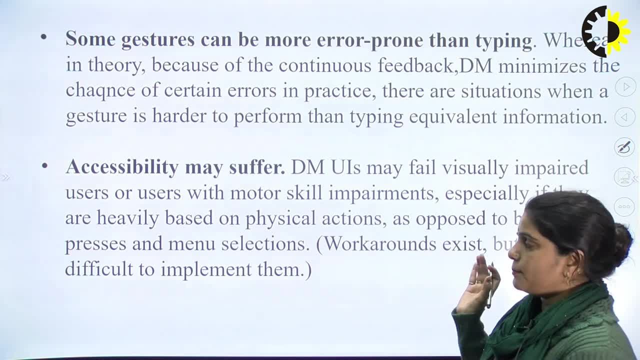 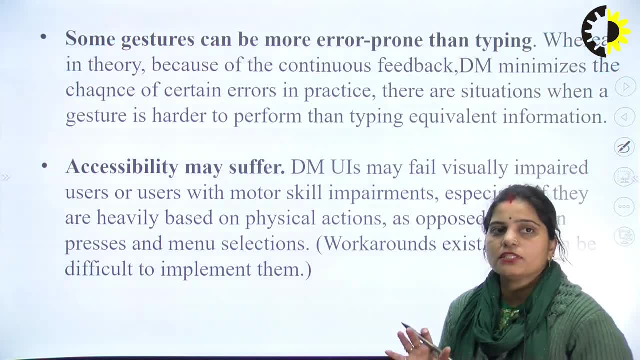 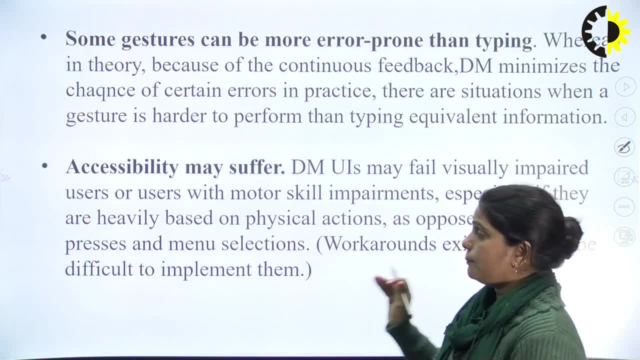 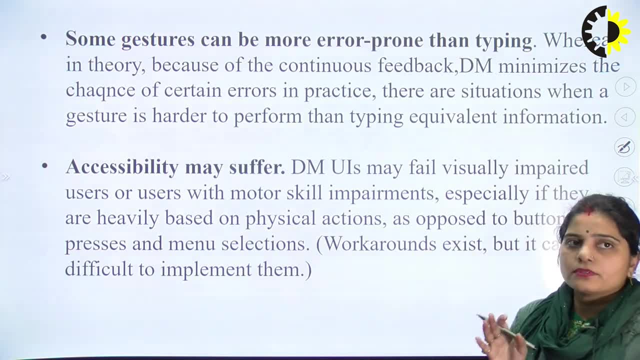 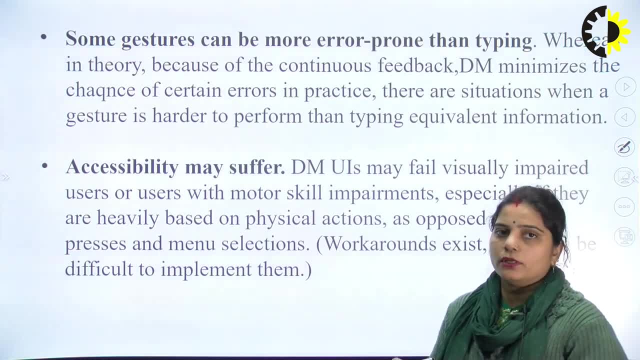 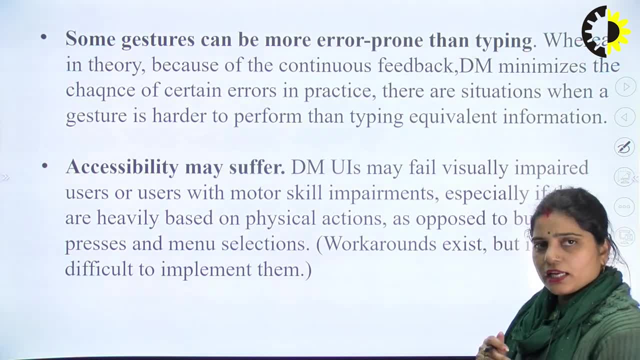 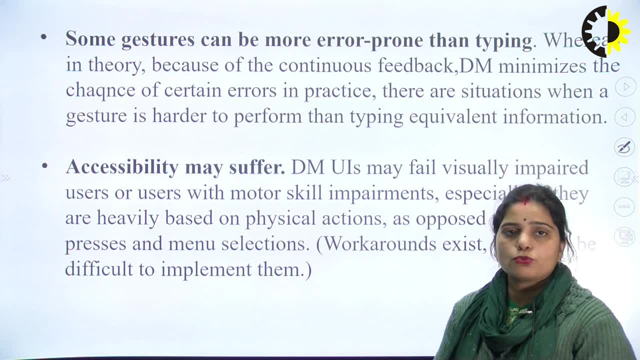 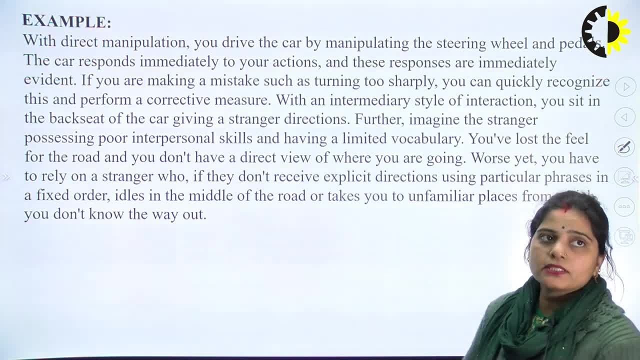 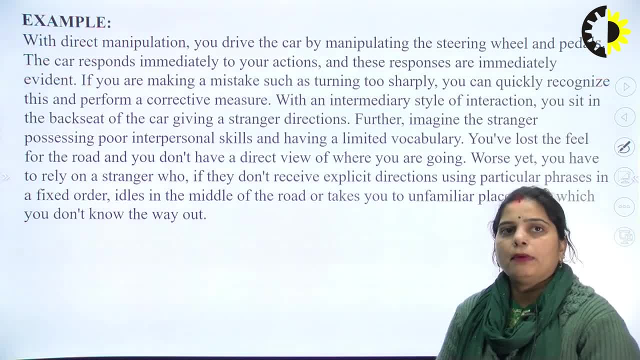 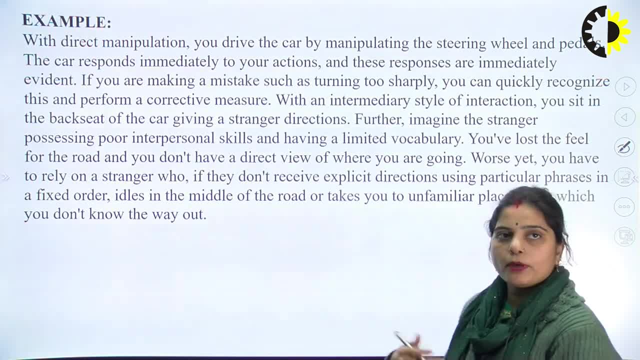 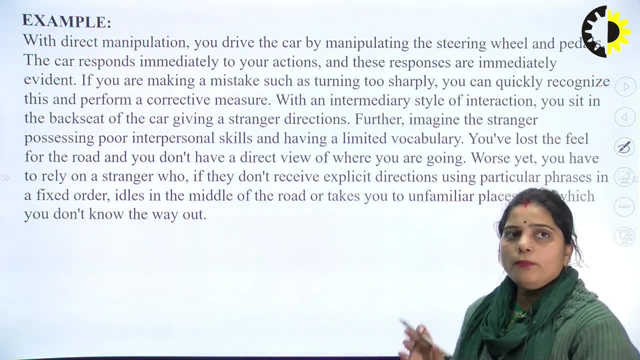 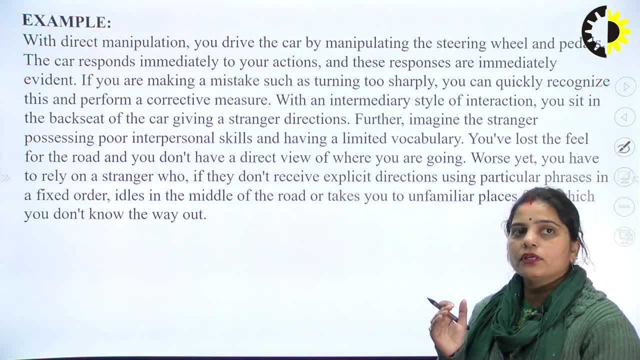 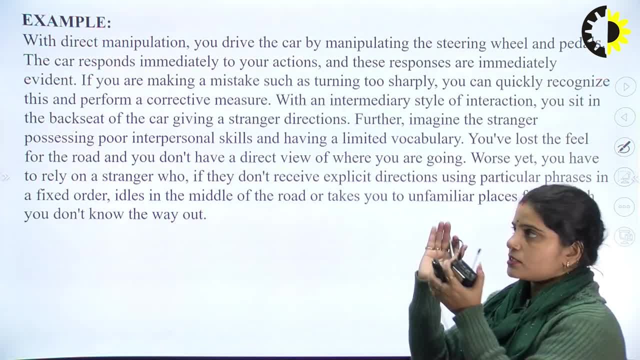 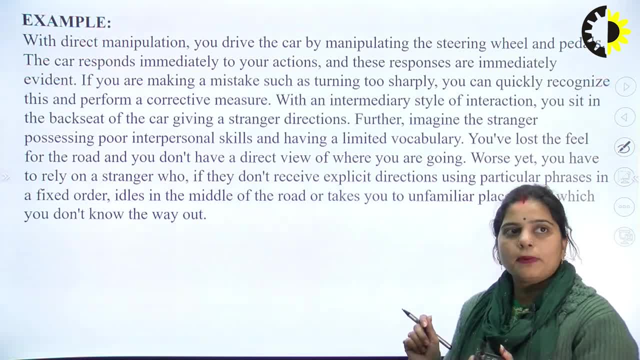 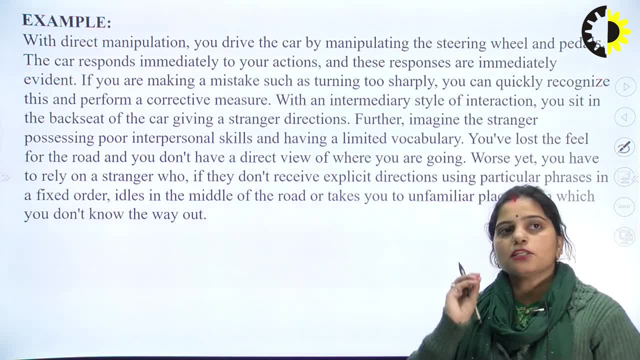 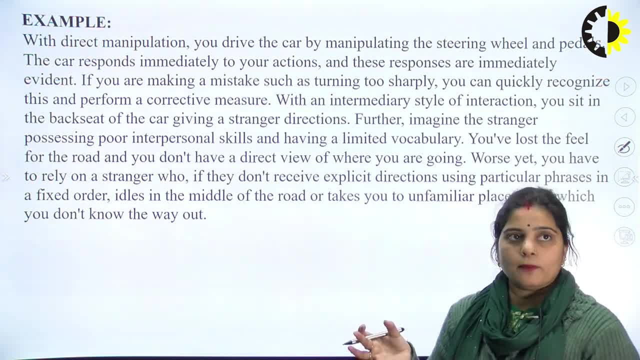 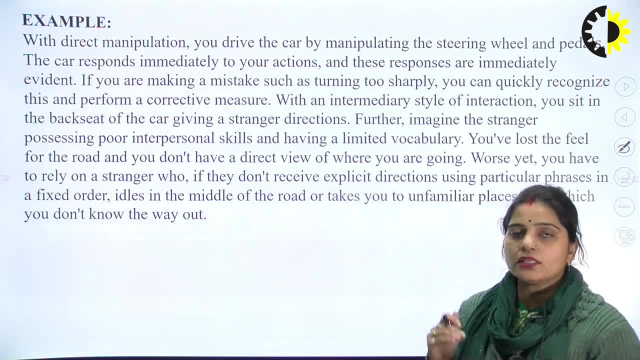 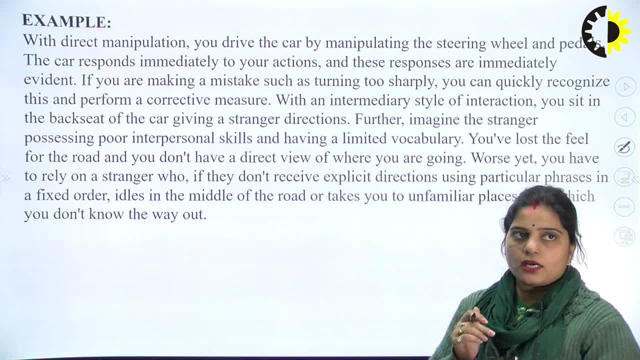 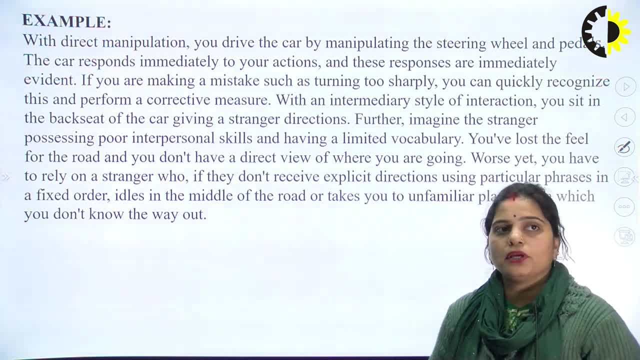 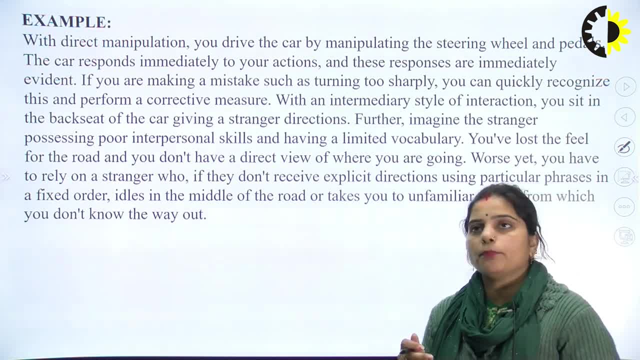 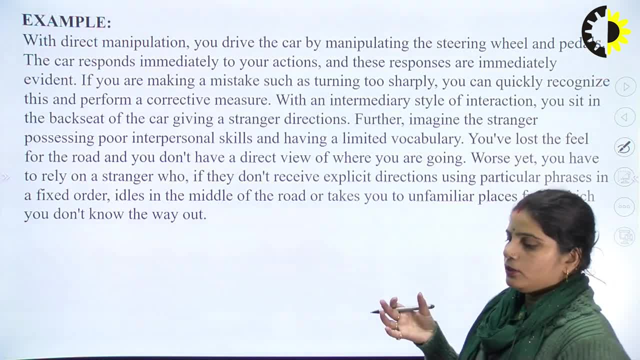 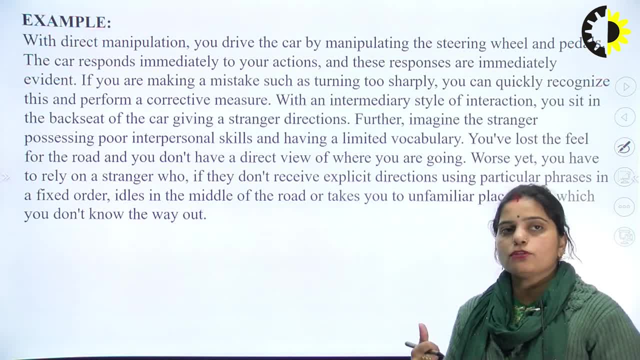 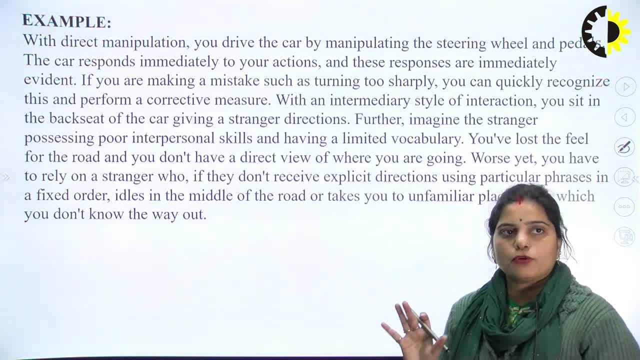 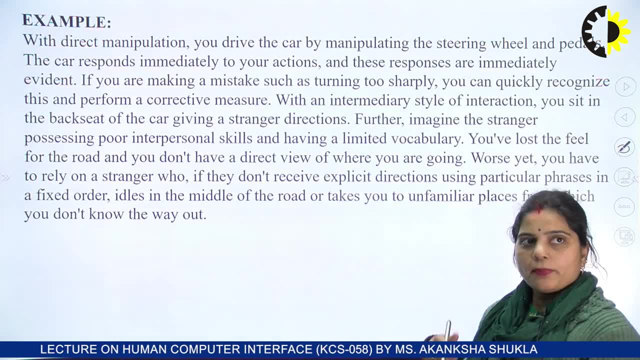 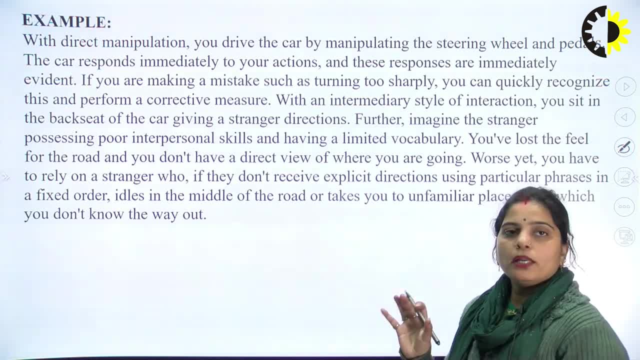 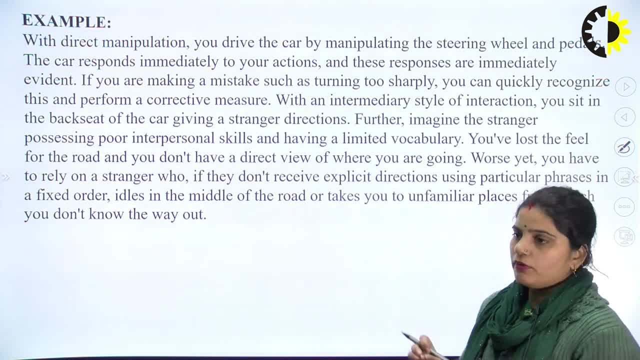 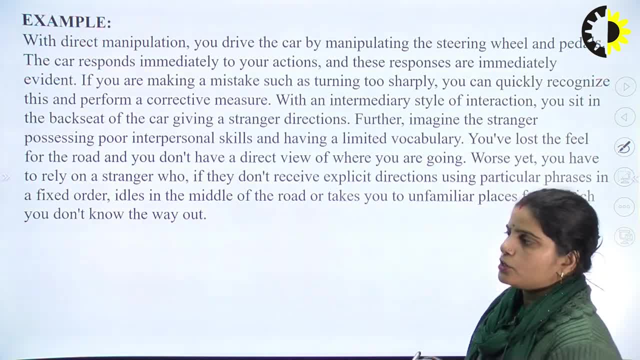 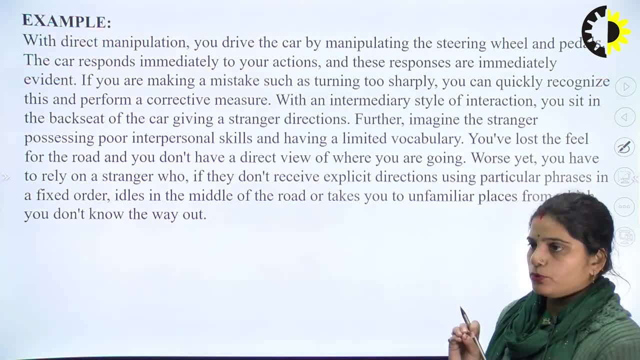 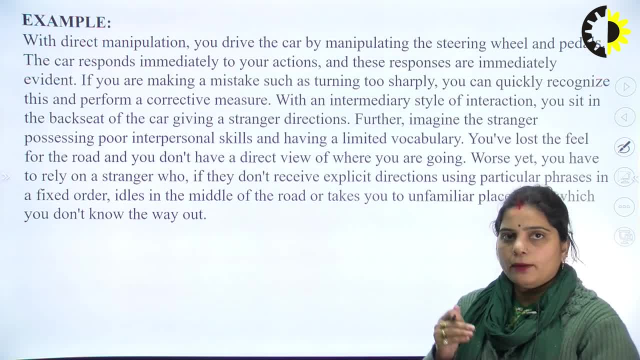 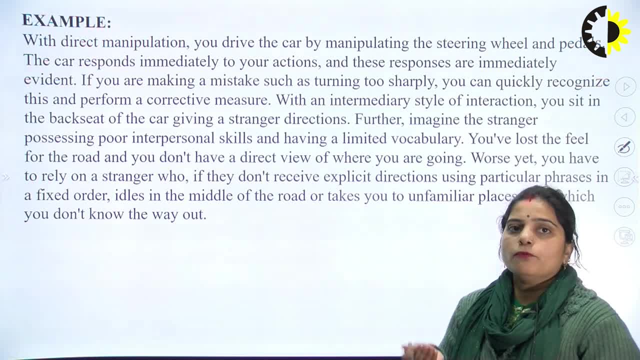 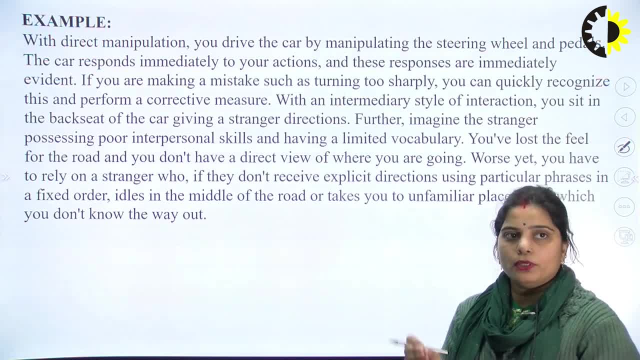 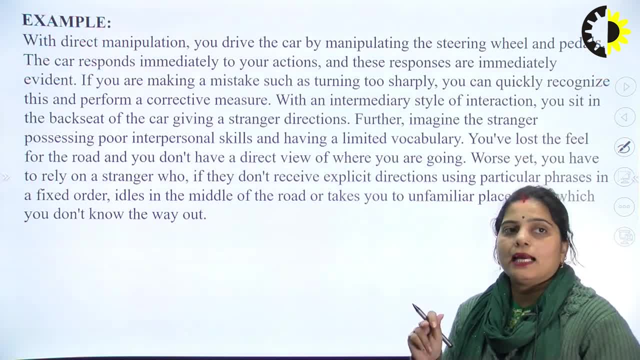 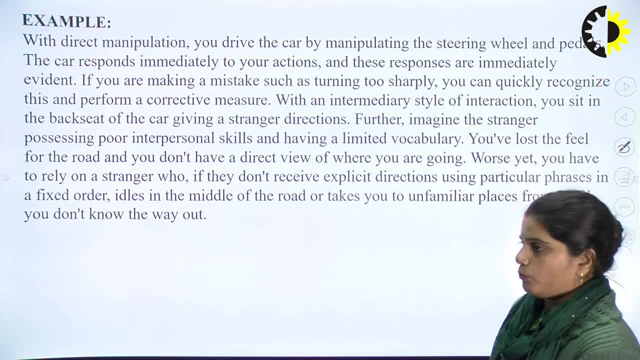 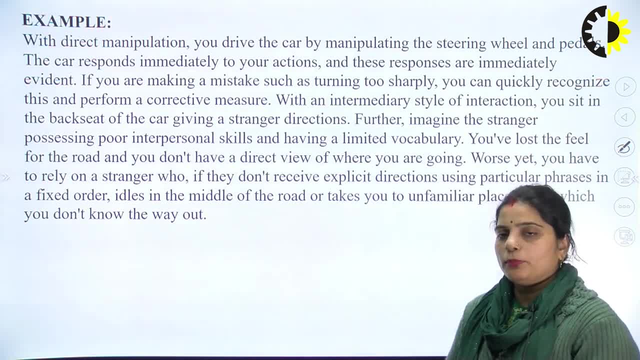 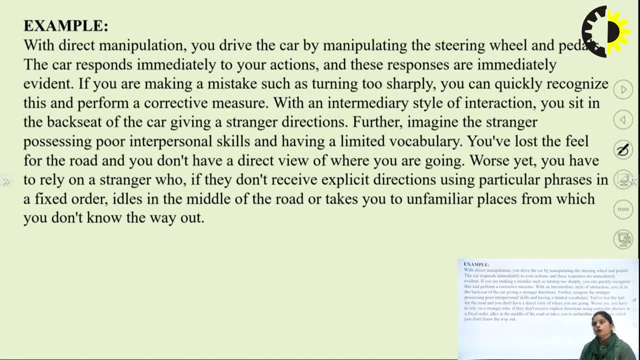 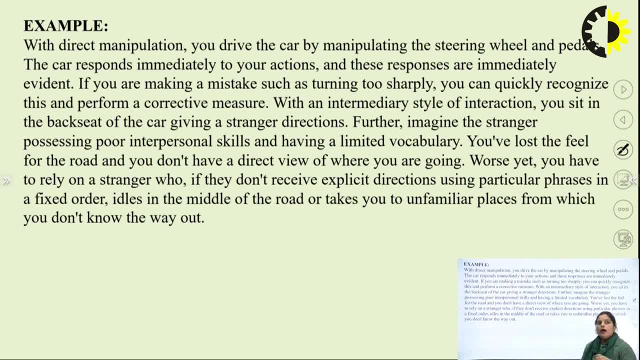 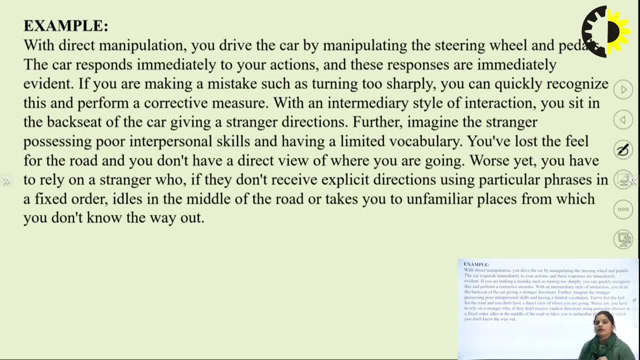 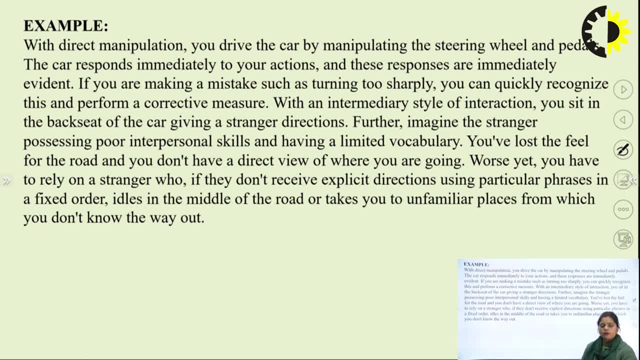 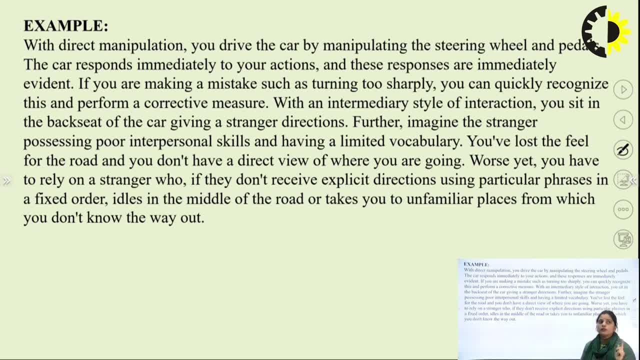 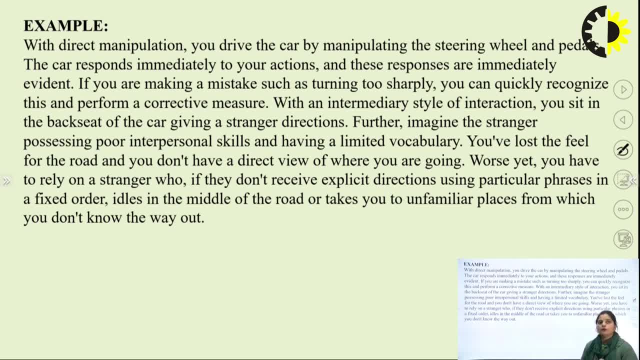 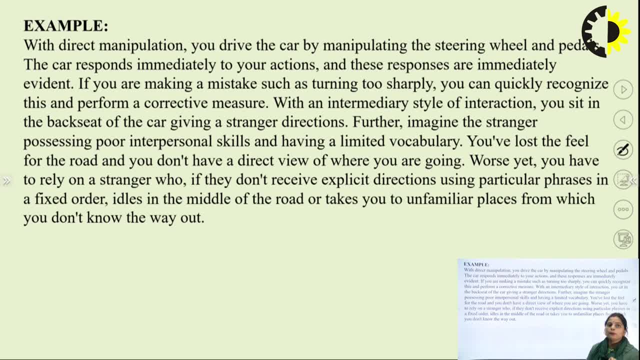 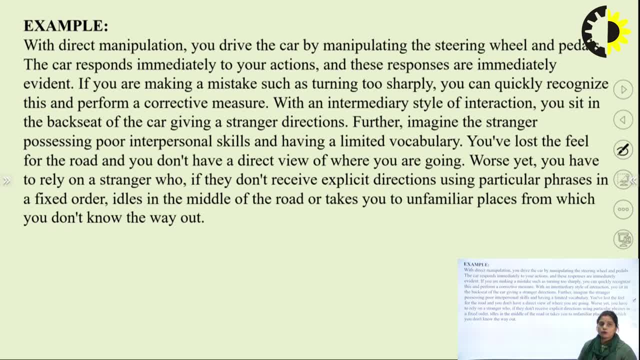 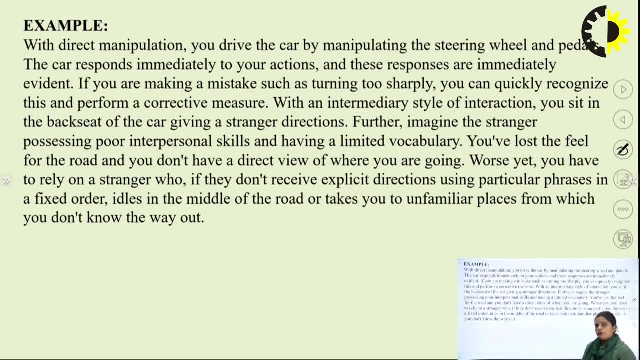 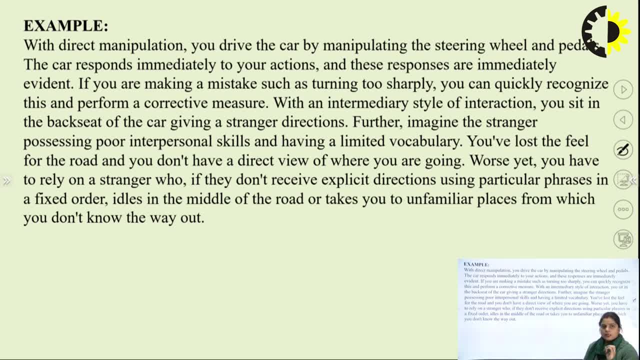 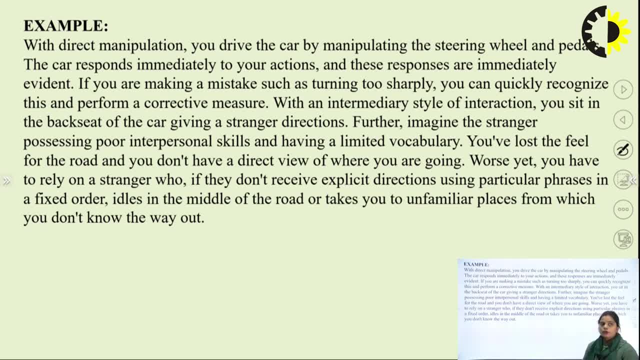 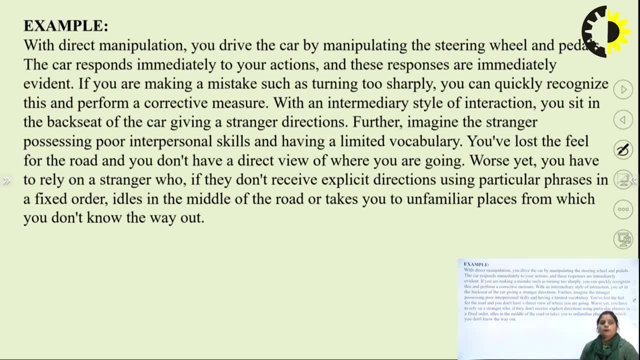 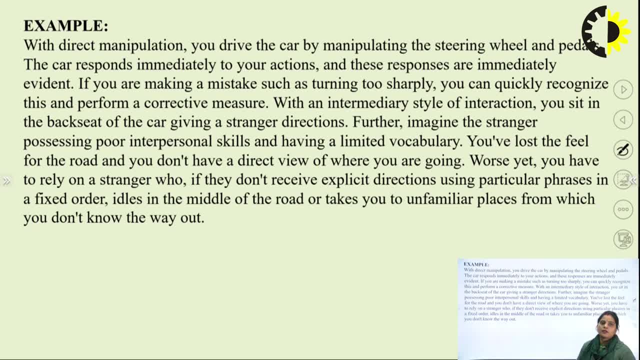 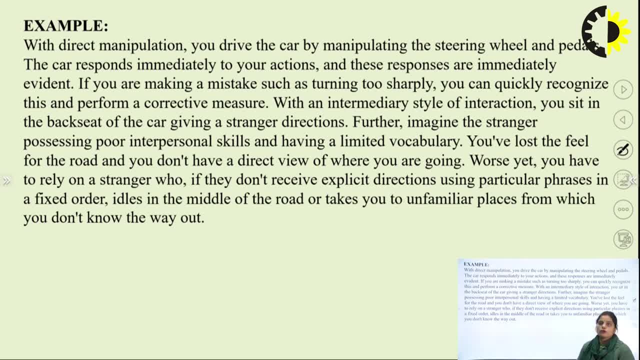 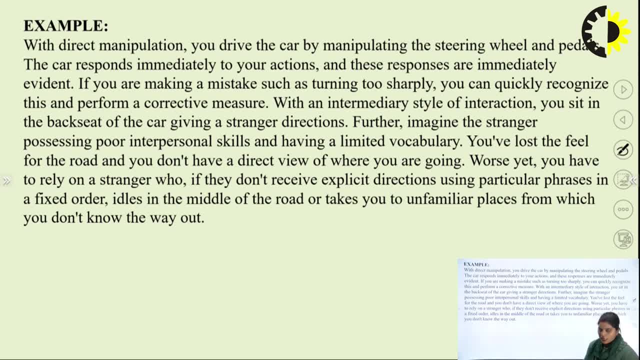 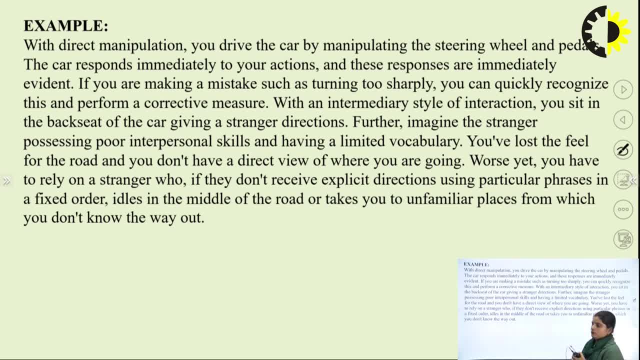 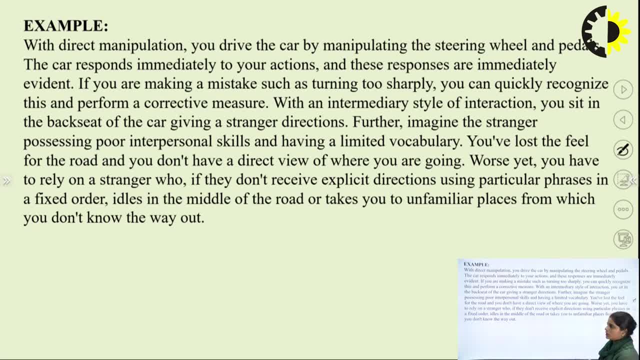 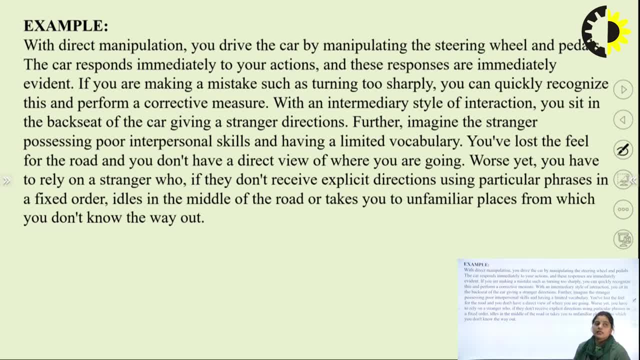 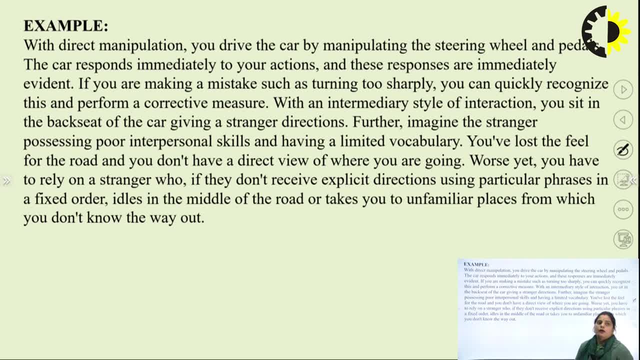 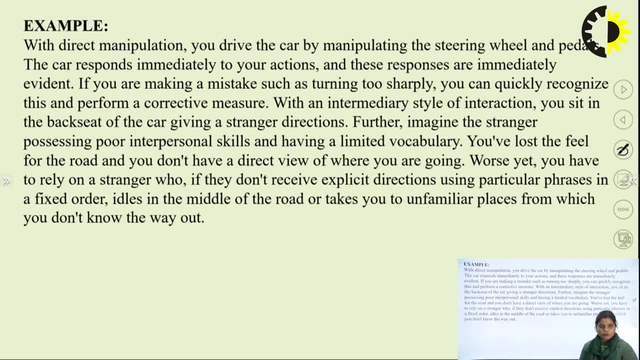 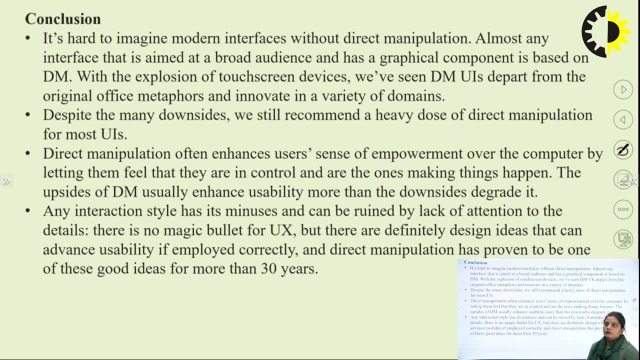 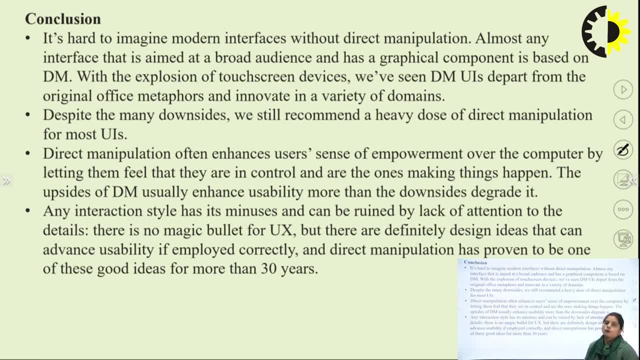 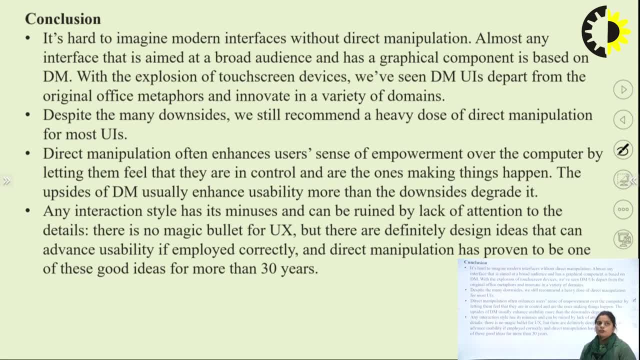 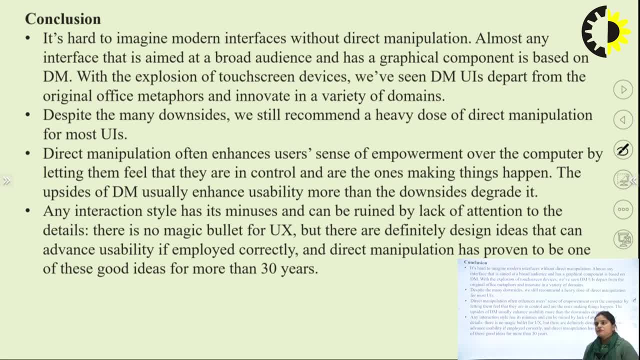 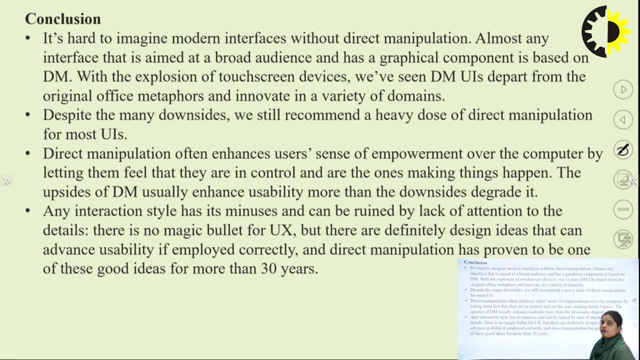 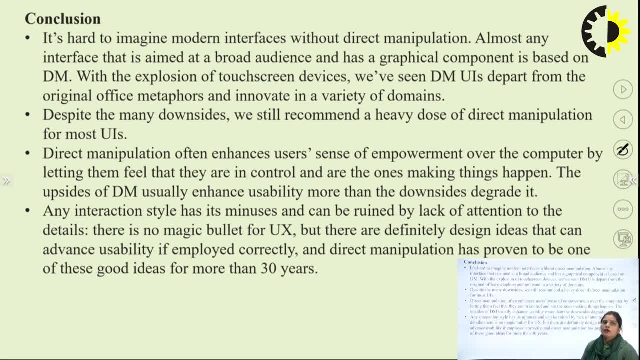 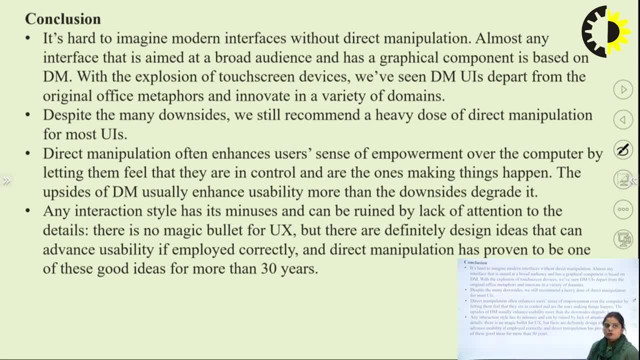 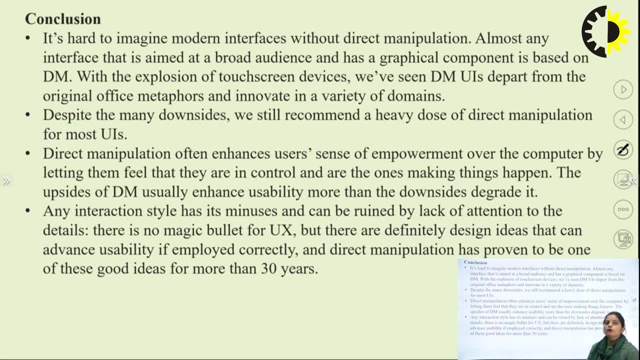 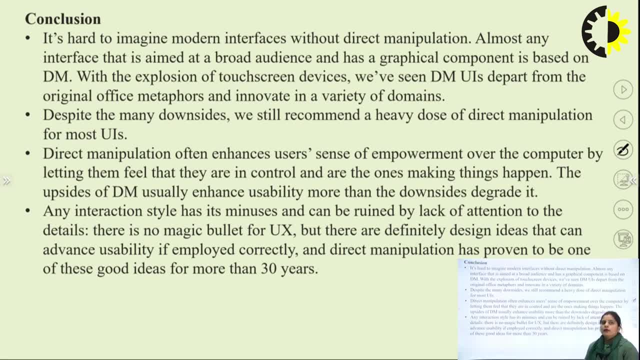 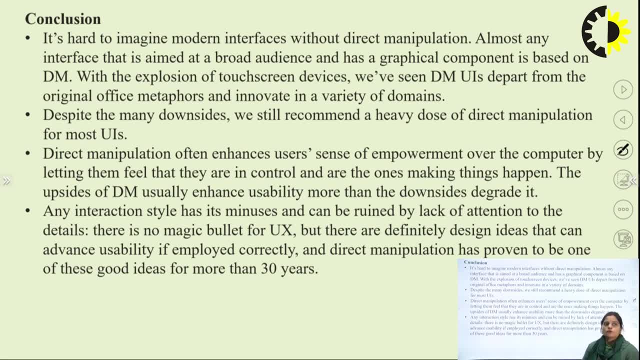 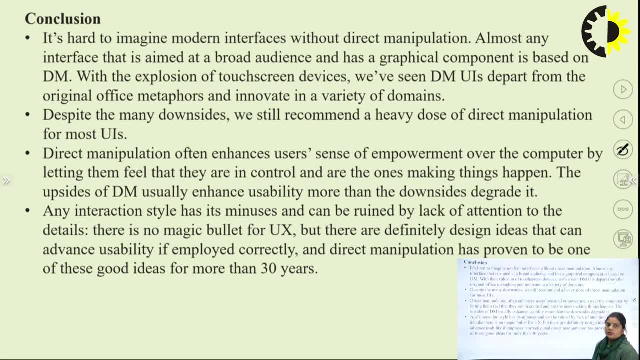 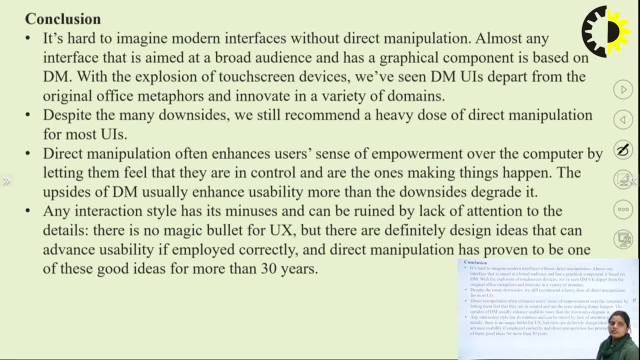 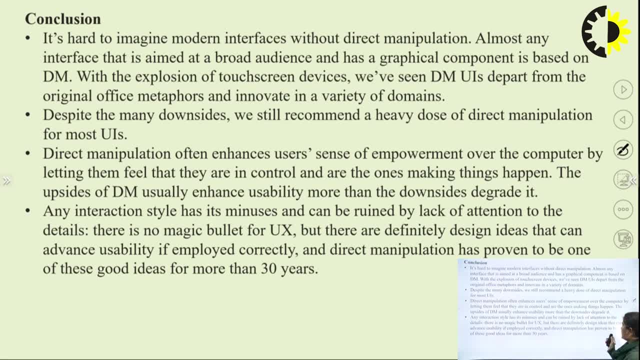 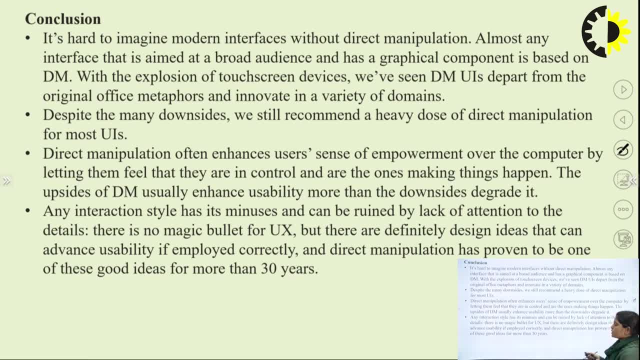 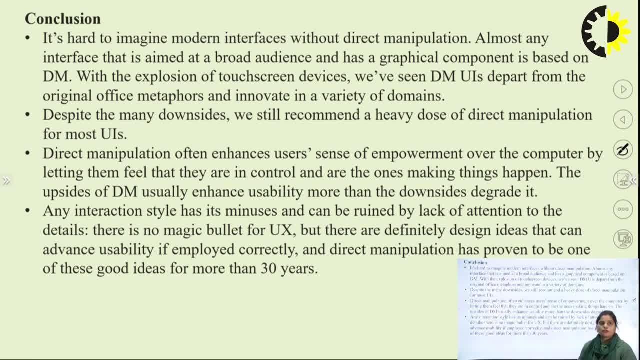 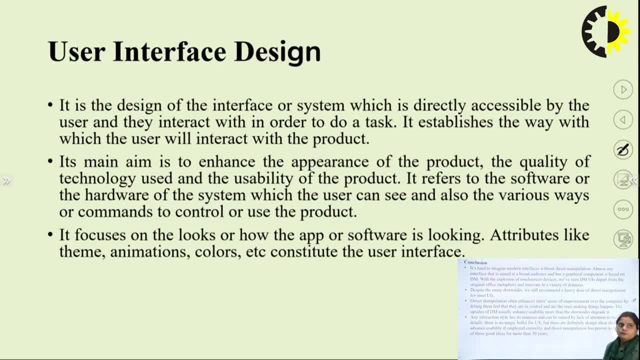 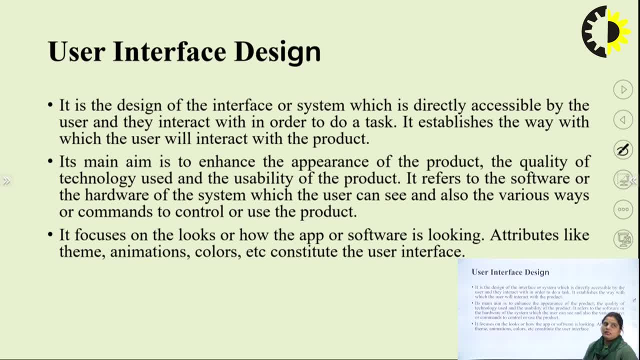 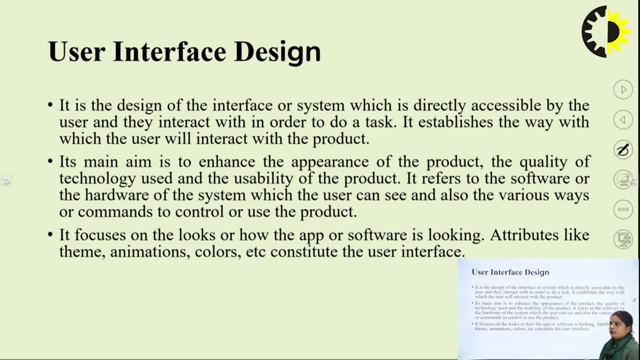 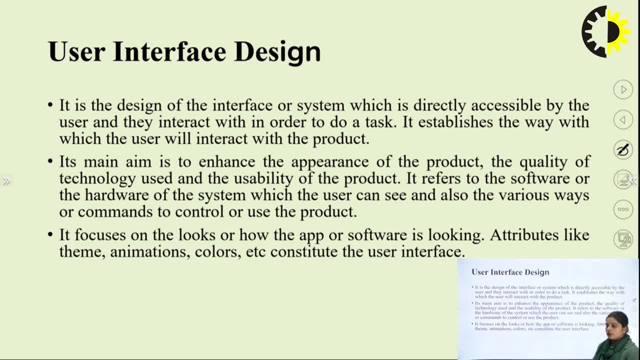 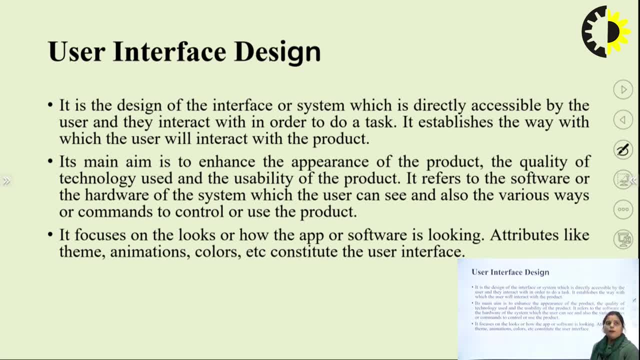 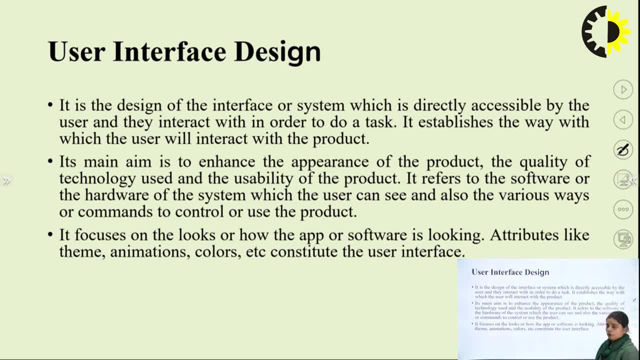 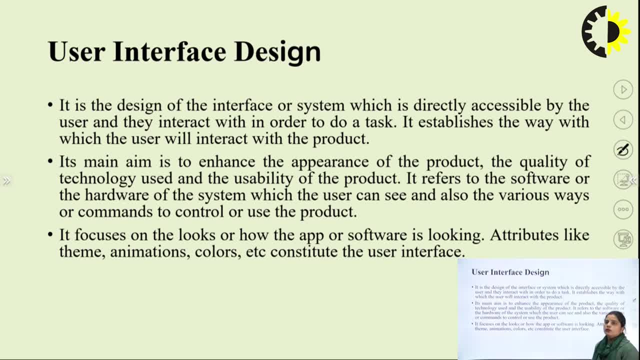 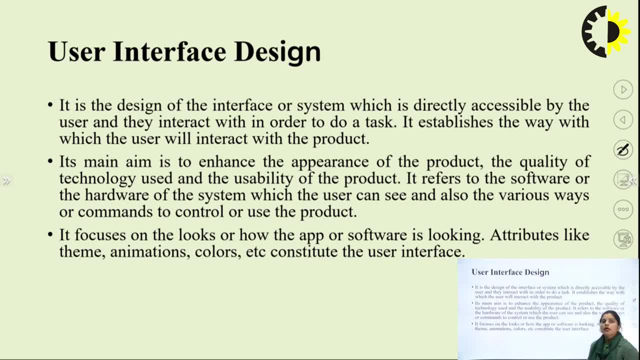 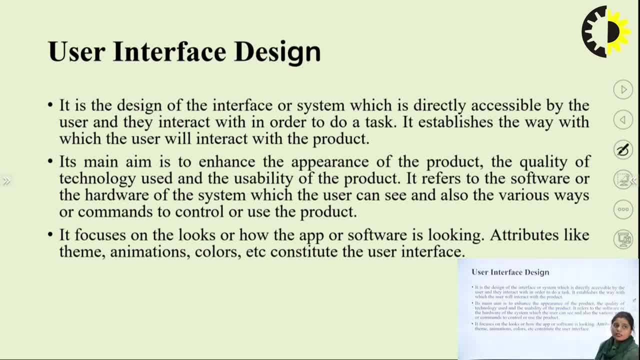 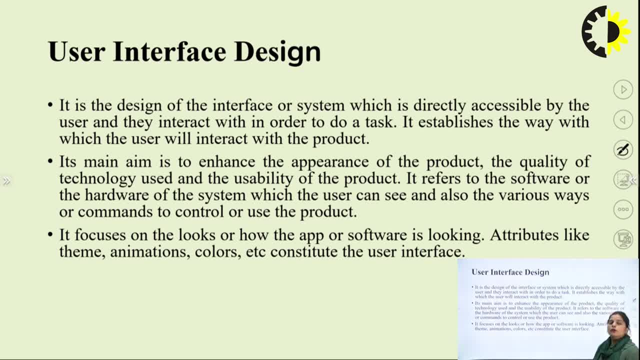 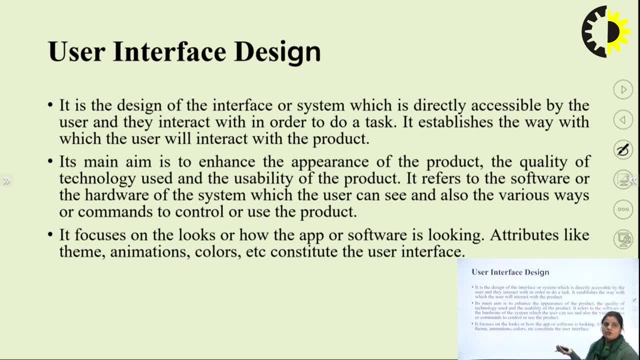 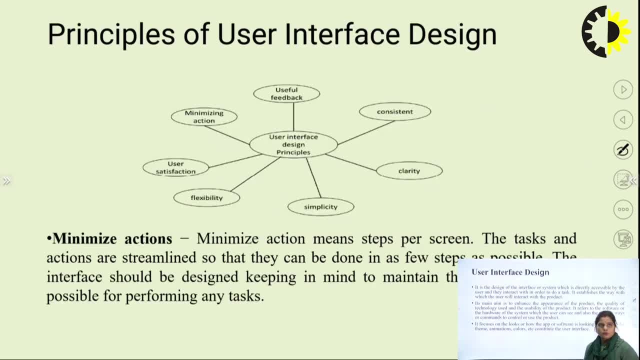 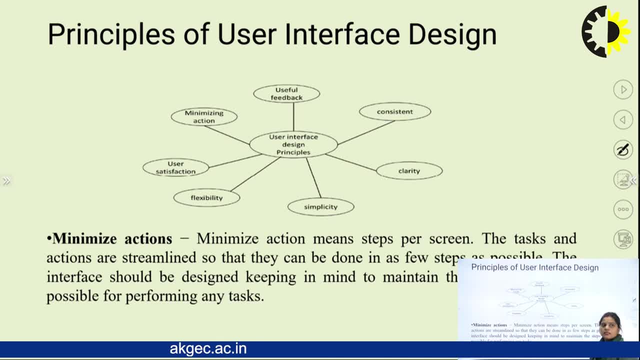 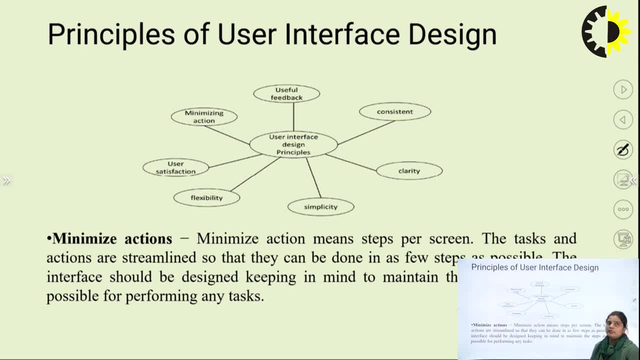 clarity, consistency. these are the some principles while designing the user interface. you have to follow these principles for designing the user interface designing so first of all. first one is: minimize the actions. minimize actions means the minimizing the steps per screen, the tasks and the actions which are streamlined. so the task and the actions should be streamlined so that they can be. 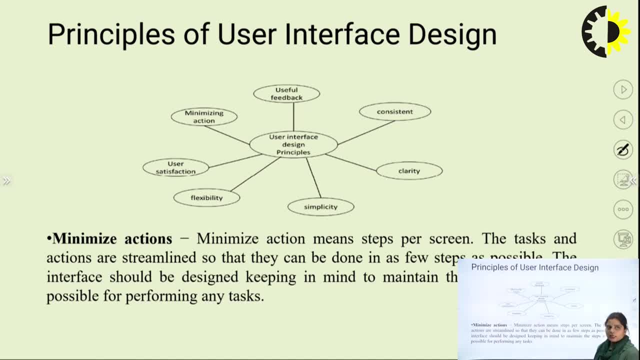 done in as few steps as possible and these can enhance, enhance the usability of the objects over these screens and the interfaces should be designed while keeping in mind to maintain these steps as few as possible for performing any task. to perform any task, the interfaces or the actions or the task should be streamlined. it should not be too large or should not be too. 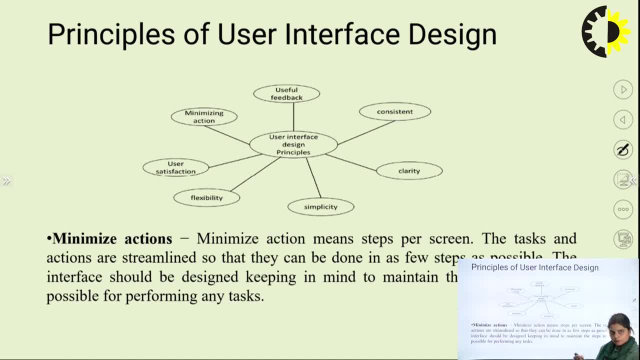 much so that it creates the bohemian inside the mindset of the person. or after some steps, suppose you have to, suppose you are going to on some, there is a machine and you have to on that machine, etc. to switch on that machine you have to follow multiple steps. so after one or two step you get. 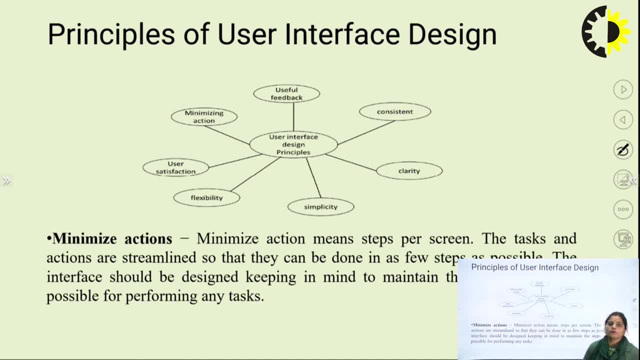 bored or is, or it may be possible that you quit from that state and you keep ideal, okay. so the actions or the tasks or the interfaces should be designed in such a manner, or should be designed keeping in mind that, to have some few steps as possible to perform any task. the second one is 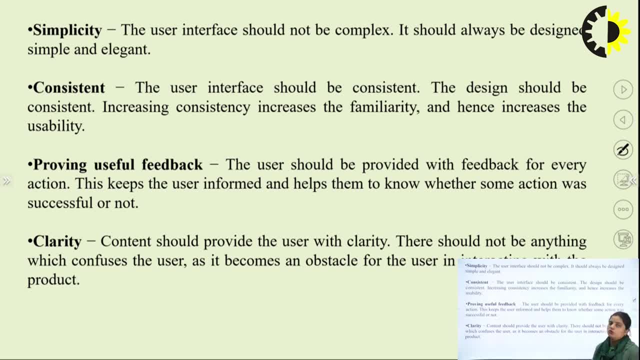 simplicity. the user interface should not be so much complex. it should always be designed in the simple and elegant manner so that the novice users can also understand what is there and what is the purpose of this, this, of this system, whatever the interfaces, what the purpose of this particular? 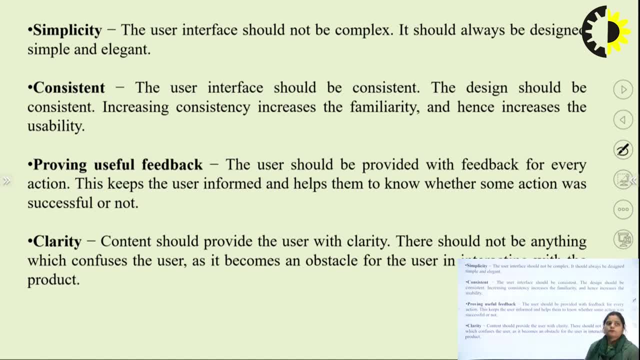 kind of system is, so it should be simple and elegant. consistency means the user interface should be consistent, means the design should be consistent. increasing consistency increases the familiarity and hence increases the usability. suppose in a system there are there are two to three sub systems, or there if there is a window, or you. 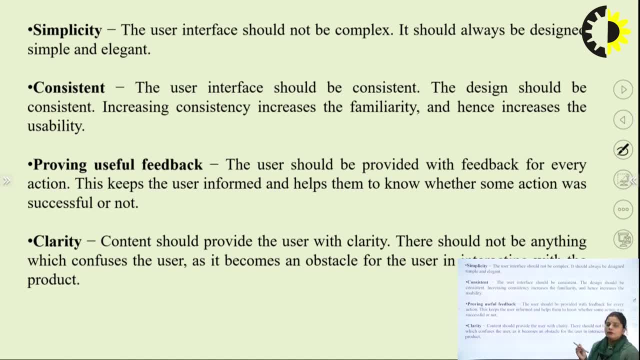 can imagine anything. so consistency should be made. consistency should be maintained in just like in the manner that, suppose you are using cross button you are using- suppose you are using cross button, you are using, Suppose, this symbol you are using to close that particular window or that particular. 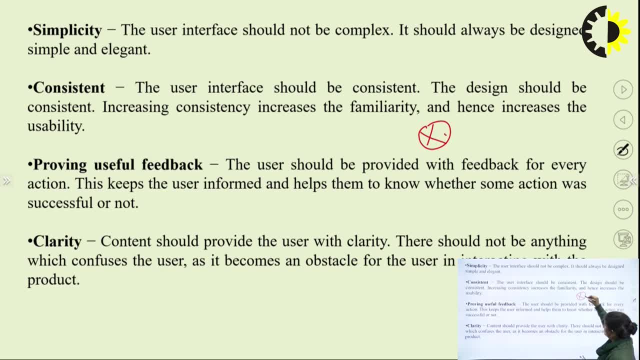 subsystem of the system. So same symbol should be used for whenever you are closing any window, any subsystem or any system, then same symbol should be used So that it does not create the confusion inside the mindset of the users that suppose you are using some places you are using this symbol, some places you are using this symbol. 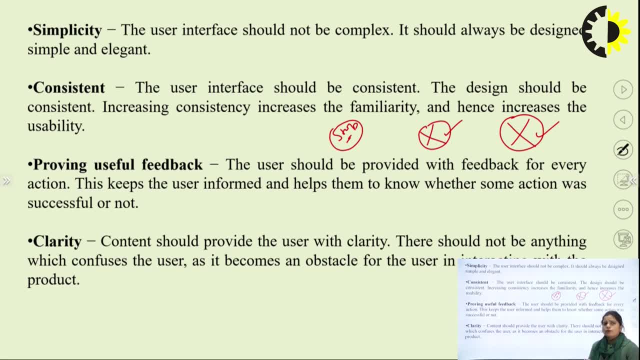 So it may distract or it may creates a confusion or or something else inside the mindset of the person. So consistency should be maintained because when you are increasing the consistency in the user interface, designing that it increases the familiarity- Suppose the person is familiar with this symbol- 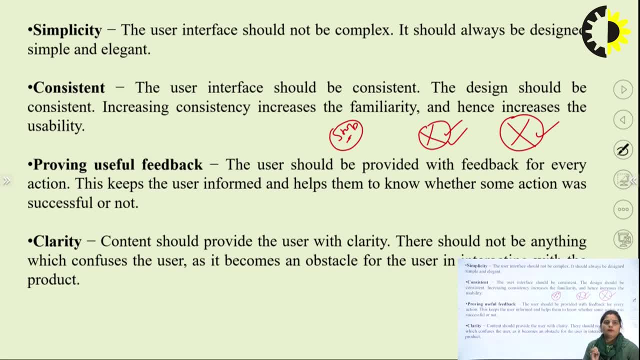 So, whenever this symbol is appears, the purpose of this symbol will be clear to him or her. only ok. So that is why this principle should be followed while designing the user interface. designing Ok Next one is proving useful, proving useful feedback, So the user should be provided the feedback for every action. 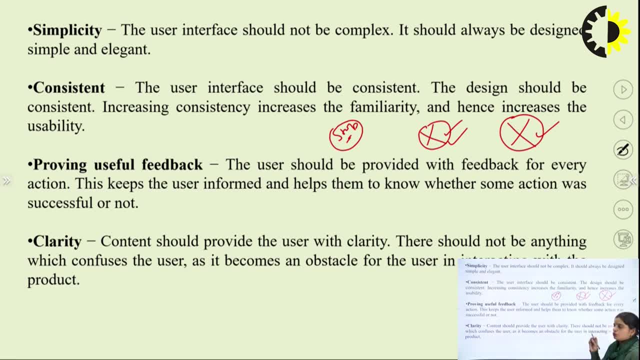 Suppose you have opened the system to, so you are giving an acknowledgement that now you are able to use the system or you can do whatever you want over the system. So at each and every action the user should be given a proper feedback. ok. 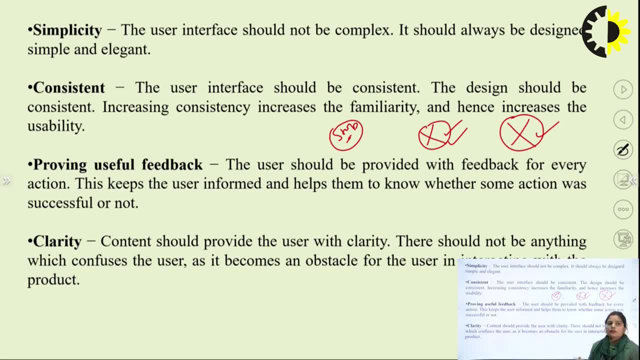 This keeps the user informed and it helps the users to know whether the some action was successful or not. Suppose you have logged in successfully, then then a message or acknowledgement should be appeared over the screen that you have logged in successfully. So these kind of feedbacks help the users, or these informations help the users in keeping. 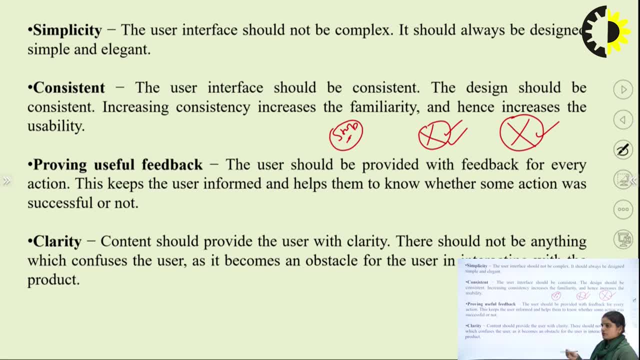 their mind that whether he is performing the actions, some action, whether he had performed some, whether he had performed that action successfully or not. The next one is clarity. So the content should provide the user proper clarity. There should not be any confusion, Ok. 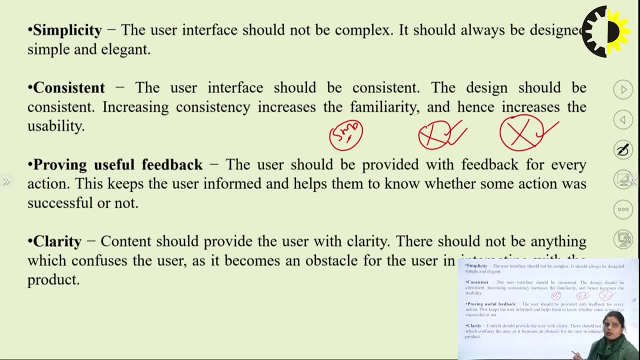 Ok, ambiguity, or there should not be any confusions? okay, as if there will be. if there exists some- uh, the confusions, or some disturbance, then it becomes an obstacle for the user in interacting with that product. so there should be proper clarity or the the things. whatever you are. 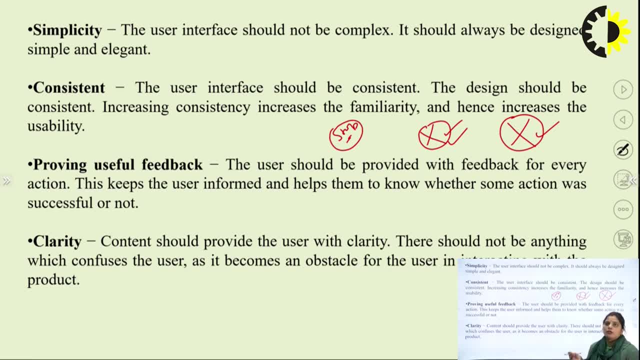 writing, or whether you are displaying any message, whether you are displaying any text. these things should be, these things should be represented or should be presented with proper clarity, with the use of simple and clear words. not so much complex word should be used here, because if forever for 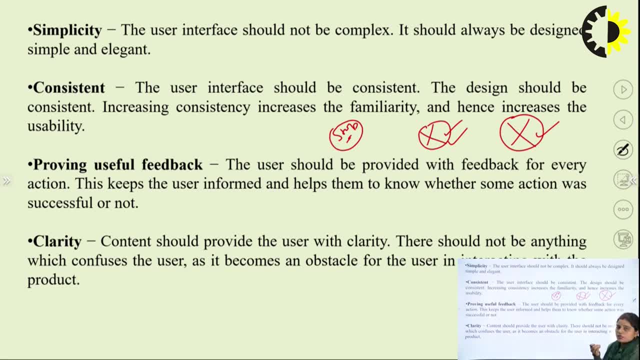 example, if a novice user is using that interface design or that system is used by the novice user, then it may be possible that that technical word should not be known to him or her. so it become, it becomes obstacle or it becomes problems for that particular user that he is not aware with this word. so whatever the content you are providing, it should be. 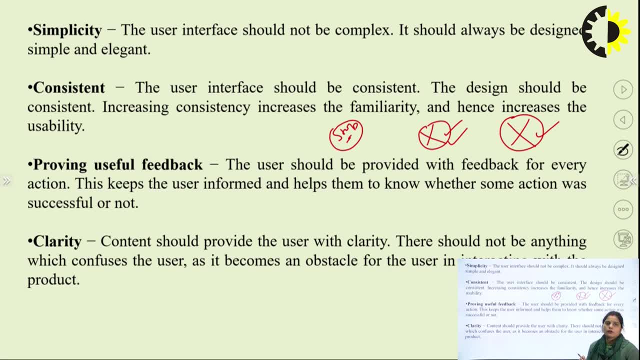 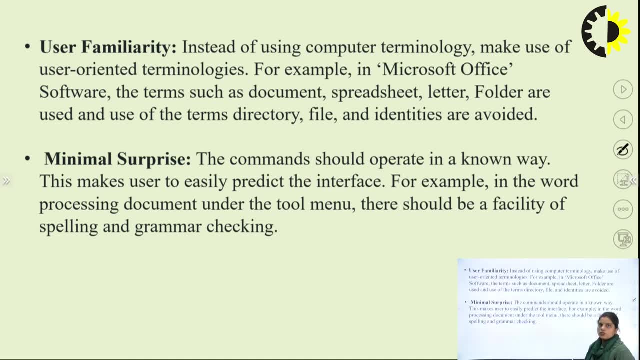 very much clear and it should be not complex now: user familiarity. instead of using the computer terminologies, or instead of using too much complex or too much technical words, make use of the user oriented terminologies. for example, here the example is given that in microsoft office software the terms such as document express sheet letter. 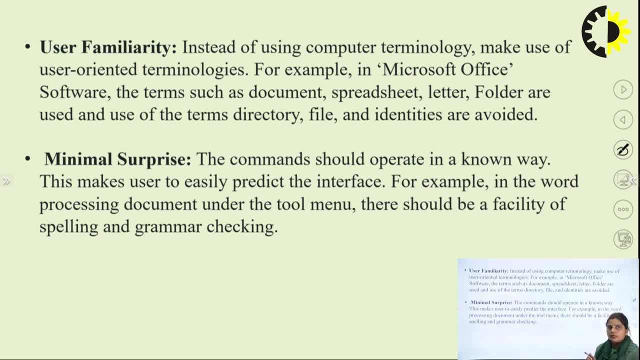 use of the terms directly, files and identities are avoided because these words are sometimes in terms of computer terminologies which the persons are not the from. with these words the persons are not too much familiar. so that's why in the microsoft office, the software, the terms such 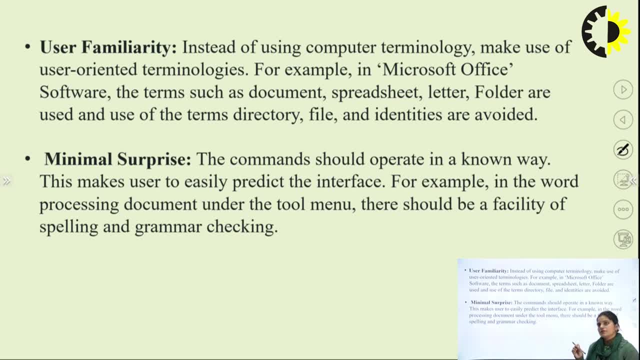 as document, spreadsheet, letter folders are used because these terms are too much familiar in comparatively to directory file identity. okay, so that's why these terms are avoided and these terms of these words now minimal surprises. the command should operate in a known way. this makes the users to easily predict the interfaces, just like an example in the word processing document under. 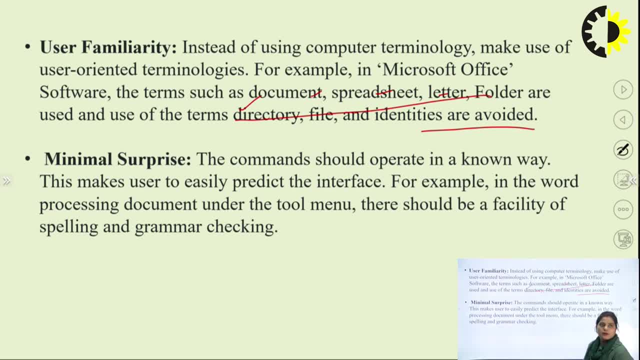 the tool menu there should be a facility of spelling and grammar checking. okay, so these options can, or these options can help the users in checking the grammars or the spellings of the documentation. so the command should be operating in a known way the operator, the command should be operated in a easy or simple manner. so by using these commands, the user. 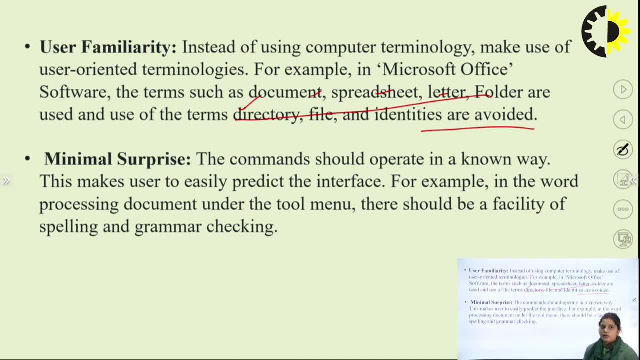 can easily predict the interfaces with the use of these commands. so these, uh, these tools or these commands or these helping features can help the user in more familiar or in more easy manner, and they can be facilitated by these kinds of commands or these kinds of buttons. next one is recoverability. the system should provide a recovering facility to the users. 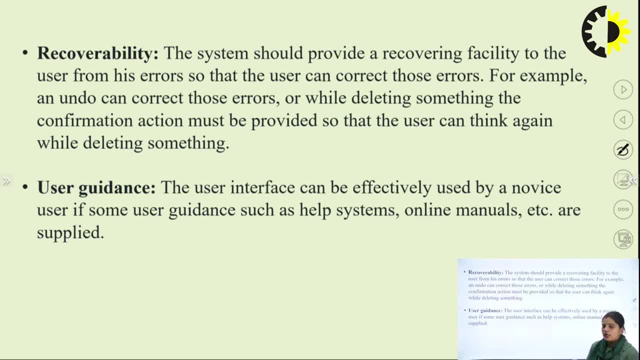 also suppose, just like, for example, a user has committed, a user has had committed a mistake. now what to do? he had committed a mistake, so there should be an option to to correct those errors also. so there should be a recovering facility for, just like you can, you you had also. 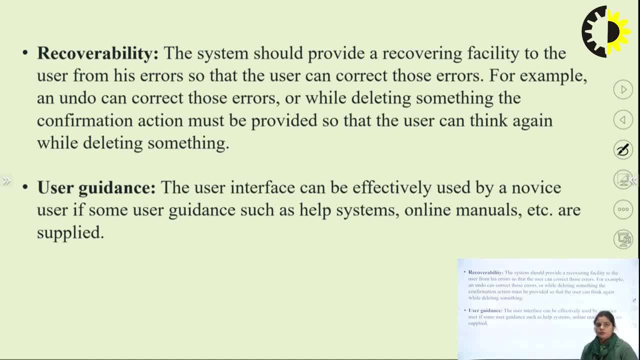 seen, or you are. you all are familiar with the undo option. okay, so what the? what is the main purpose of undo? if, uh, unknowingly, or if, by mistake, a user commits some mistake, then i'm can do, can correct those errors, or while deleting something you are, or whenever you are, deliver you are permanently. 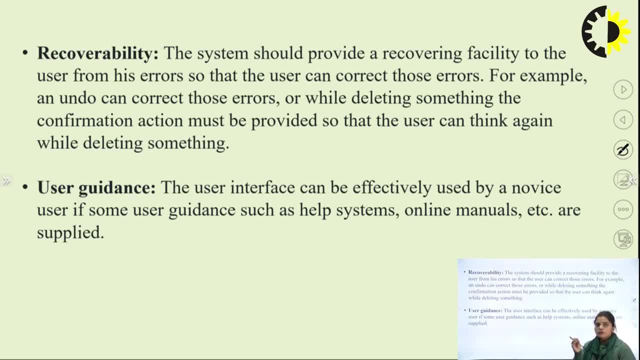 deleting any files or folders from the system. it gives you a message: okay, it give. it requires some confirmation actions from you that whether you are confirming that, whether you are permanently going to delete that file or not, so that the user can think again while deleting something. so these 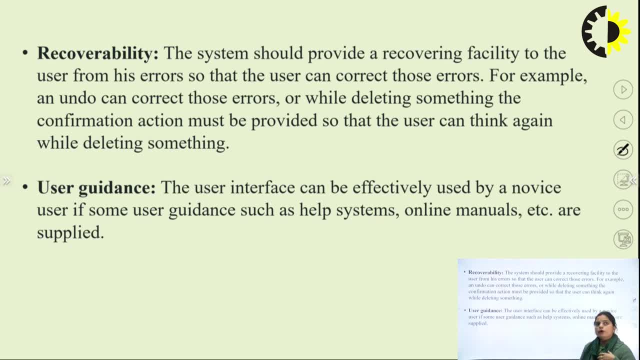 kinds of things are basically provided for, provided for this purpose only, for the purpose of recoverability. okay, so that the system should provide these kinds of options so that the person or the user can recover from unknowingly making mistakes or can also think again if he or she has. 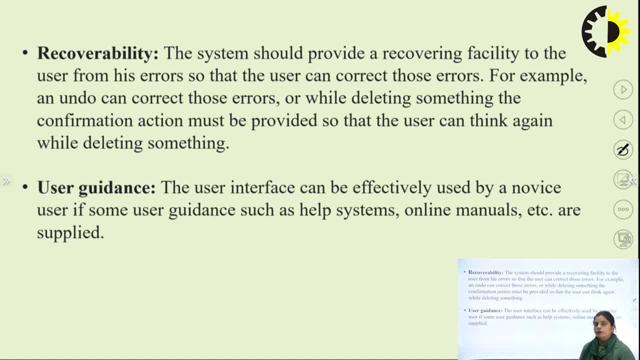 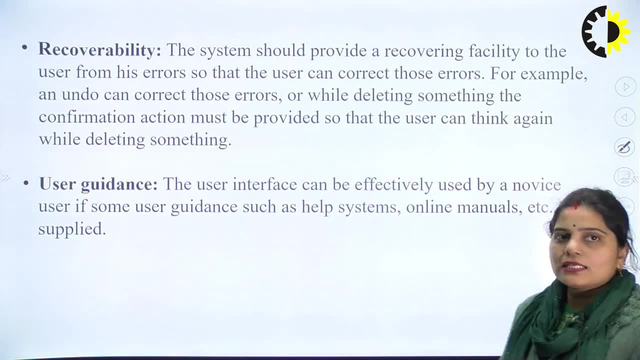 to occur him if he or she has to delete something, confirmly or not. next one is user guidance. the user interface can be effectively used by novice users if some user guidance, such as help systems, online commands and are supplied. means if suppose, for suppose a system is going to be first time used by a by any user, suppose this user is a novice user. 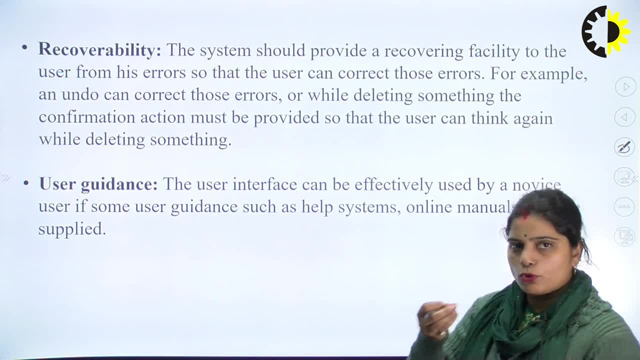 he is not familiar. he is not, uh, not um so much familiar with these kinds of technologies, with these kinds of terminology. so the user guidance which i think the help option or help system is is, i think, almost available in all the systems, in all the apps and in all.